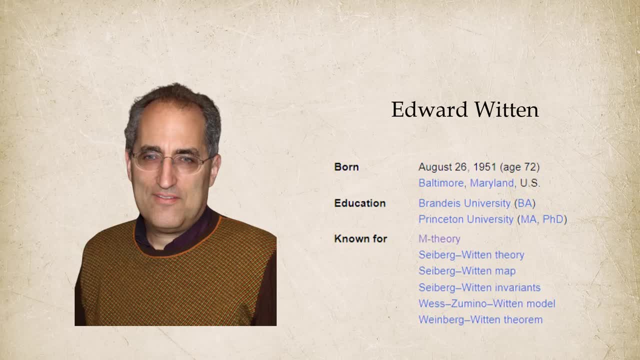 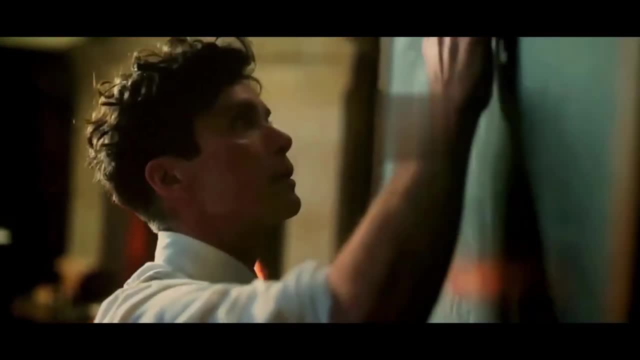 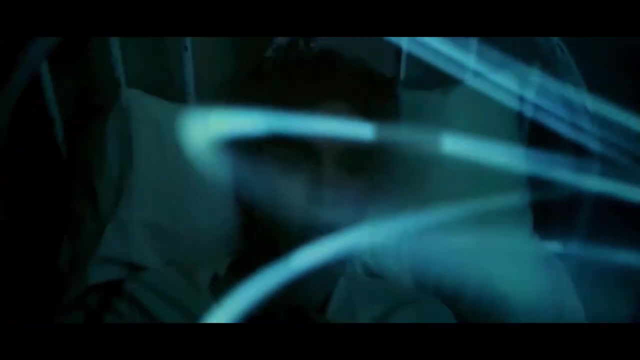 but then a very smart scientist named Witten showed that these versions are like translations of the same idea. Witten's discovery was a big deal, because it's like having five different ways to understand the same book. Sometimes one version of the theory makes it much easier to solve difficult. 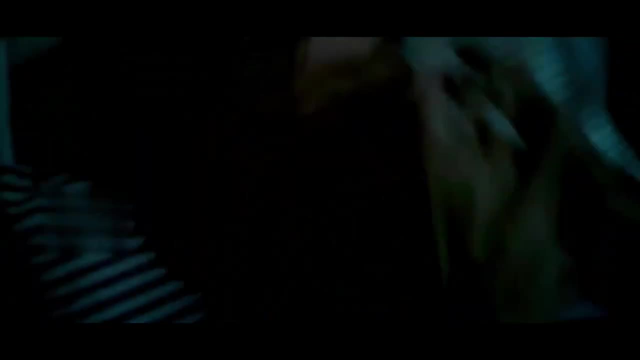 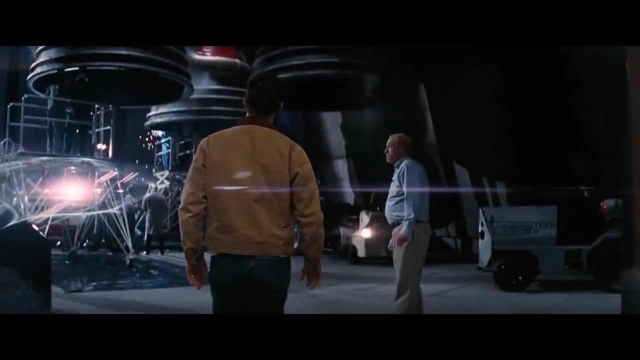 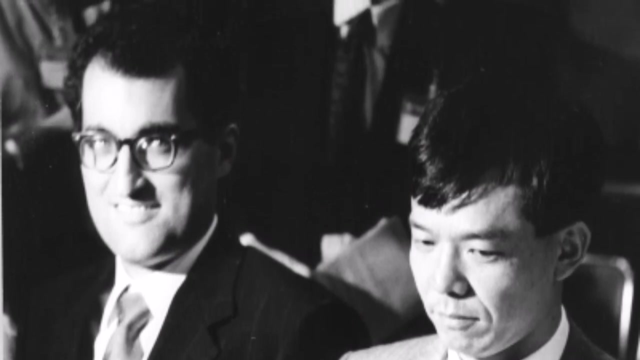 problems. So, just like different translations of a book help you understand it better, these different versions of string theory help scientists answer questions and discover new things. Witten's discovery gave scientists a powerful tool to solve difficult problems. It's called String Theory and that's why it was revolutionary. 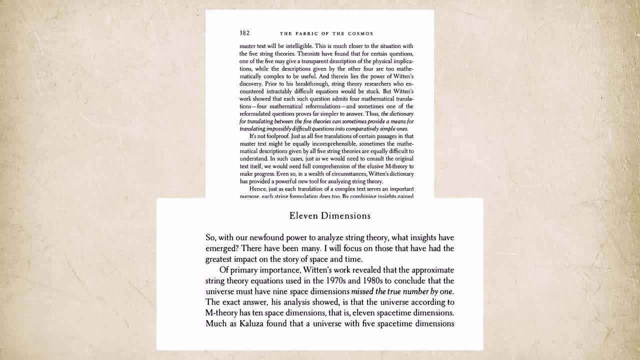 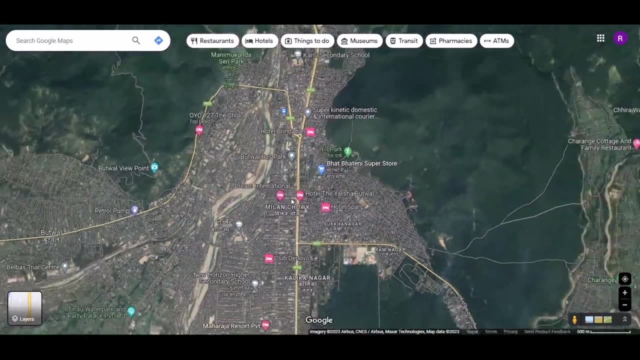 First Witten found out that the universe, according to M-theory, actually has eleven dimensions, ten for space and one for time. This was surprising, because before everyone thought there were only nine dimensions. It's like thinking there are five separate villages. 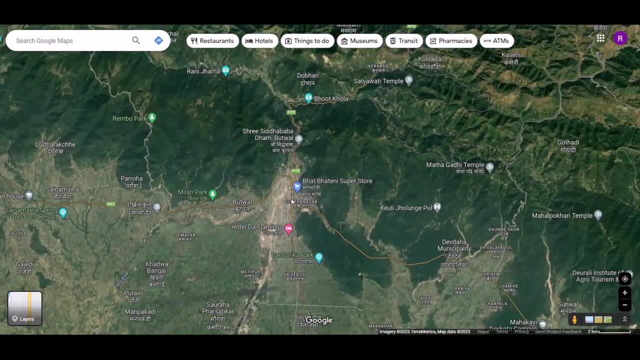 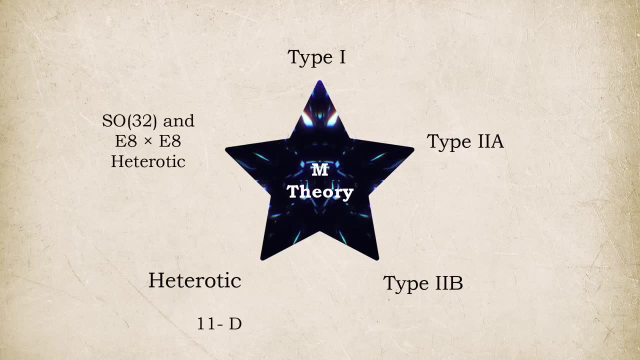 but when you look from a mountaintop you see they are all connected by roads. Similarly, Witten's analysis showed that all five string theories are connected through this extra dimension. This discovery was a big deal because it challenged what we thought we knew about. 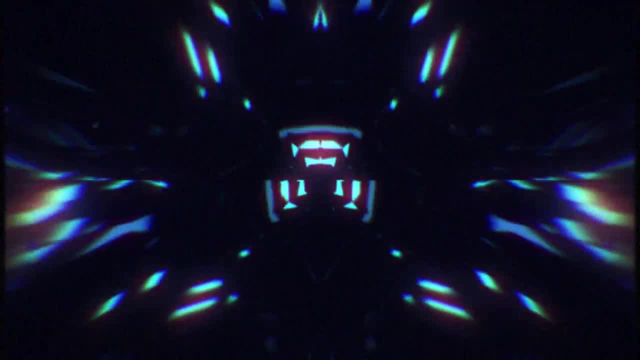 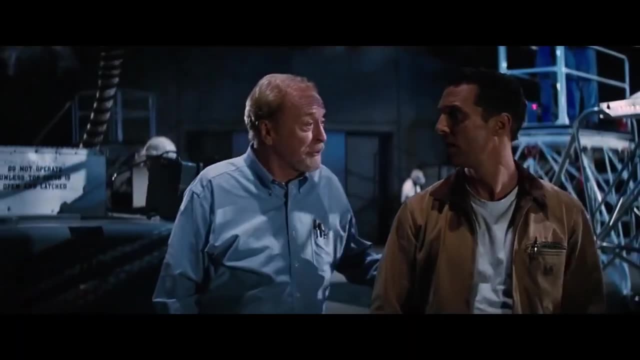 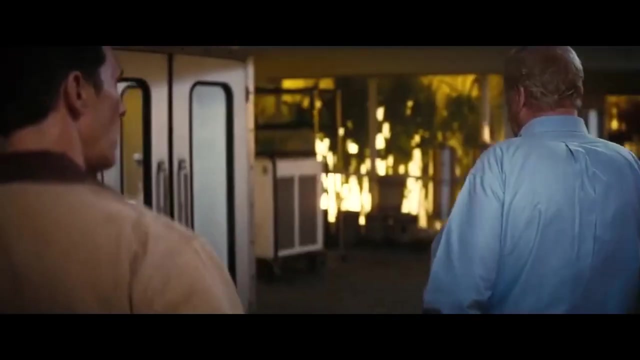 string theory. It turned out that previous calculations had missed this extra dimension because it was assumed to be very tiny, smaller than the others, But Witten's new insights showed that it was there all along. You might wonder if this changes everything we knew about string theory. In most cases, 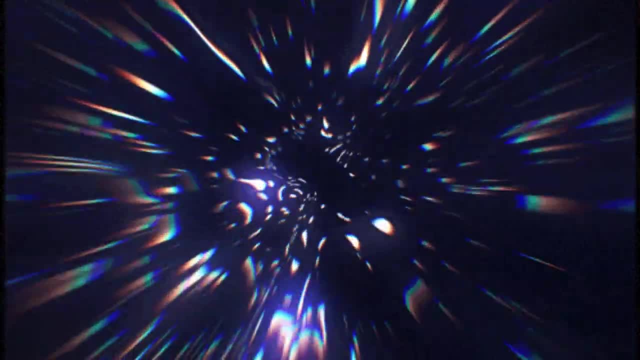 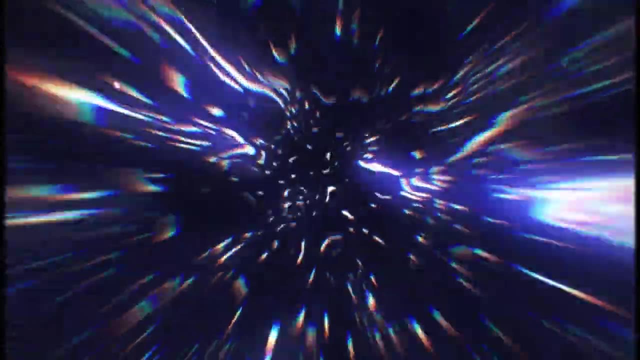 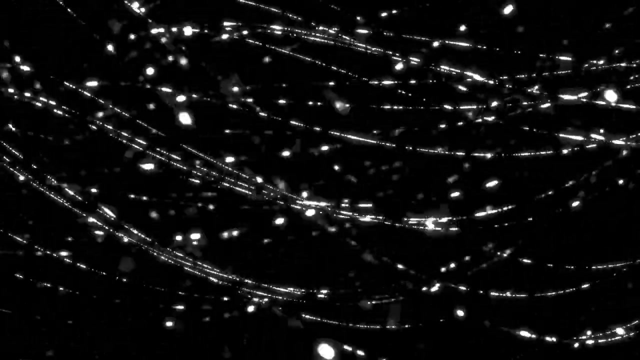 it doesn't. The new dimension added an unexpected twist to the theory, but previous work still holds if this extra dimension turns out to be very small, as we once thought. Scientists are now investigating the possibility that this dimension might not be as small as we. 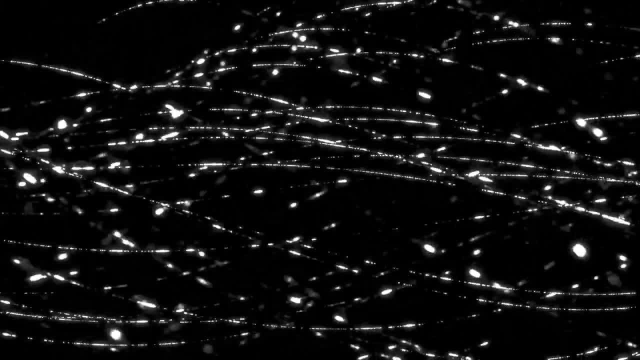 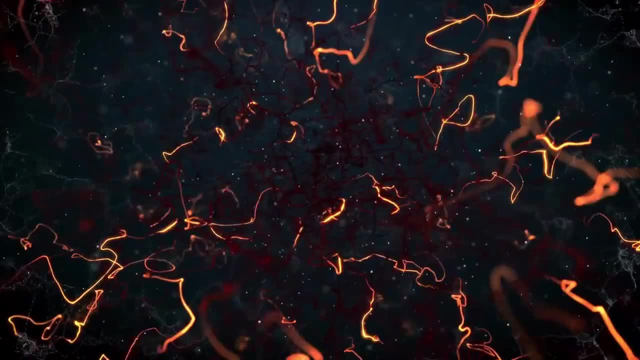 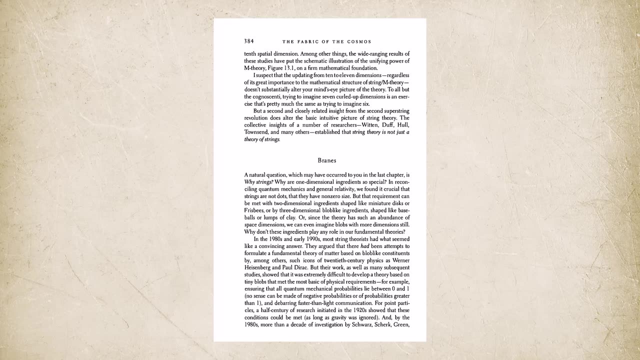 thought, and this has led to more discoveries. Another important insight from this discovery is that string theory is not just about strings, as the name suggests. It's about much more, and scientists are still exploring its full potential. Why are we talking about strings in science? What makes these one-dimensional things so? 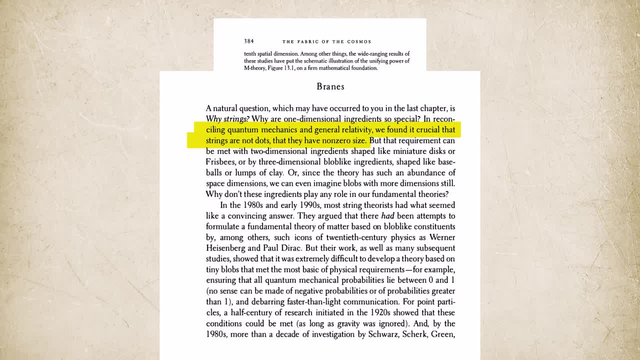 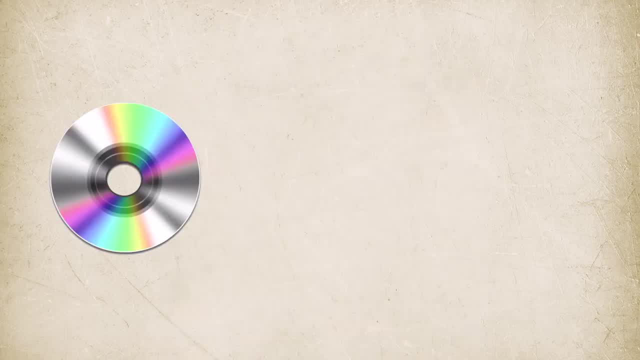 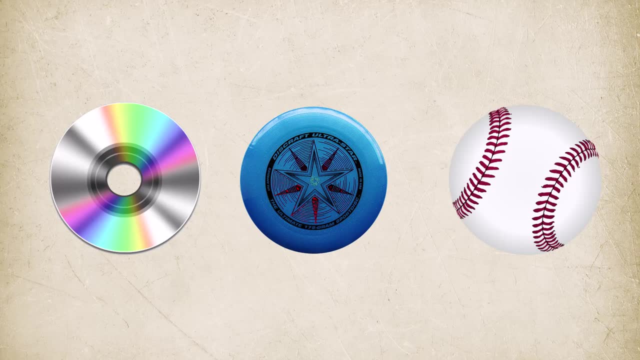 special. Well, when we tried to combine quantum mechanics and general relativity, we needed something with size, not just dots. We could have used two-dimensional shapes like mini-discs or frisbees, or even three-dimensional blob-like shapes like baseballs. In fact we have so. 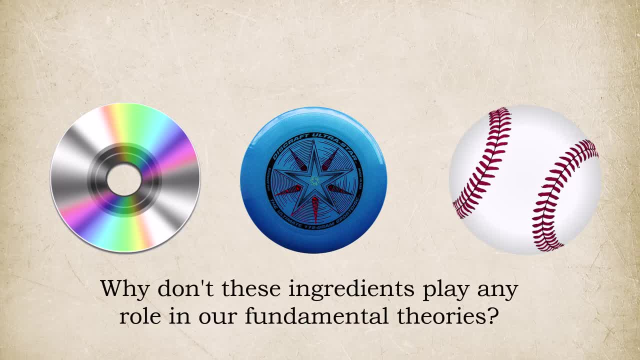 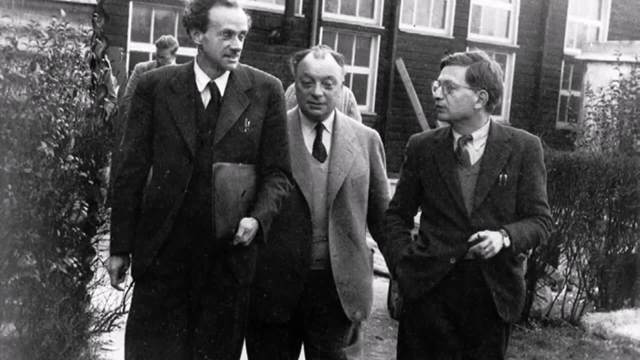 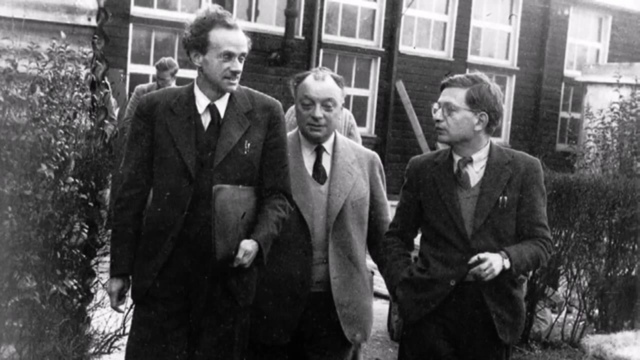 many dimensions in this theory that we don't even know what they are. So why did we stick with strings? Back in the 1980s and early 1990s, most scientists thought they had a good reason. They believed that trying to create a theory using blob-like ingredients, like Werner Heisenberg and Paul 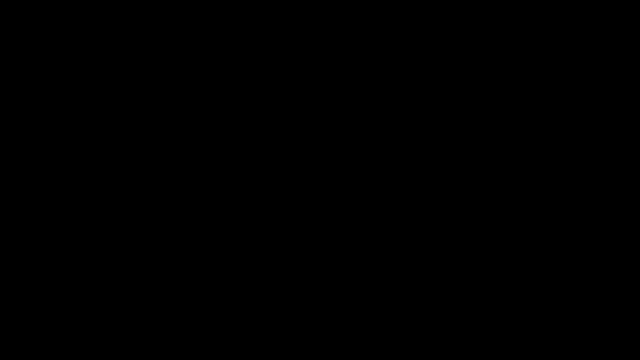 Dirac had tried was really tough. They found it challenging to meet some basic requirements like making sure all probabilities in the theory stay between zero and one. They also argued that when we were in a particle like a十-dimensional it was very difficult to 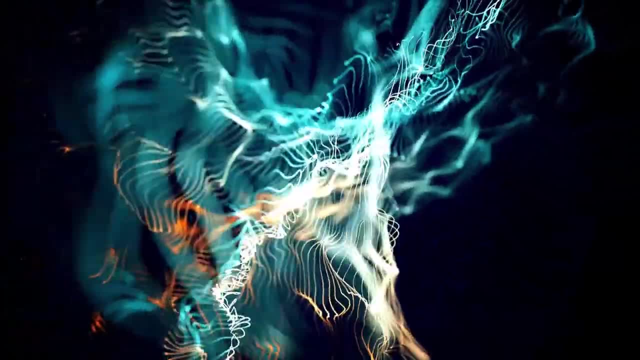 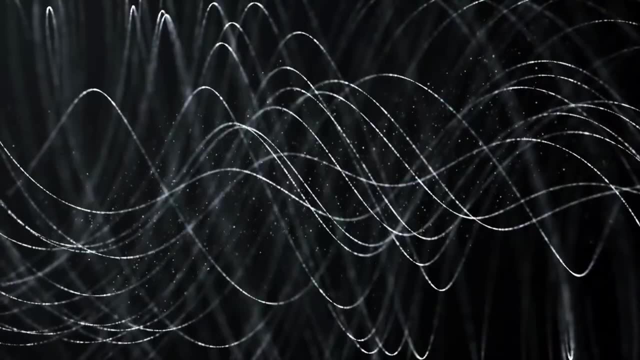 understand what was being the case in real life. When it came to point particles like dots and one-dimensional strings, things worked out surprisingly well. So researchers focused on strings, But when Witten and others showed that string theory includes more than just strings…. 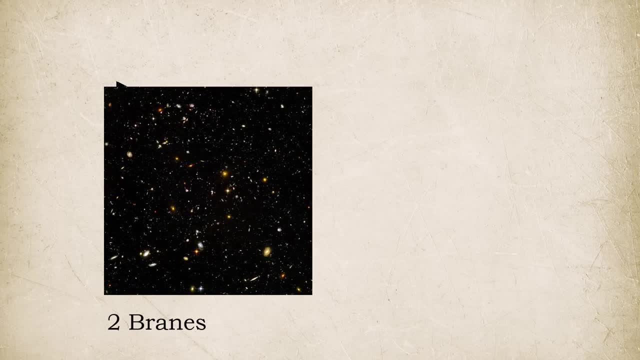 They discovered two-dimensional objects called membranes or two brains, three-dimensional objects called three brains. Even objects with more dimensions had more complex mechanisms than just strings. they were still called membranes, The Hemnahmen Fertig Positiv. Well, what's the use of creating a theory on memory more? 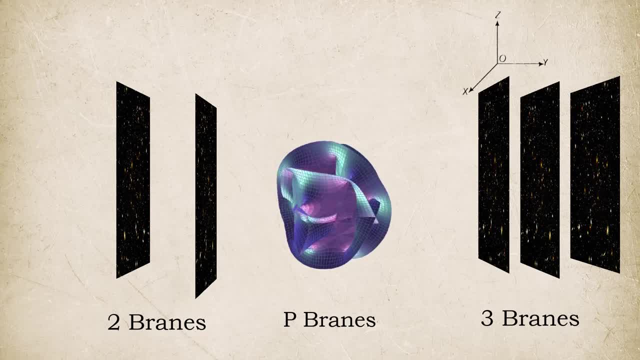 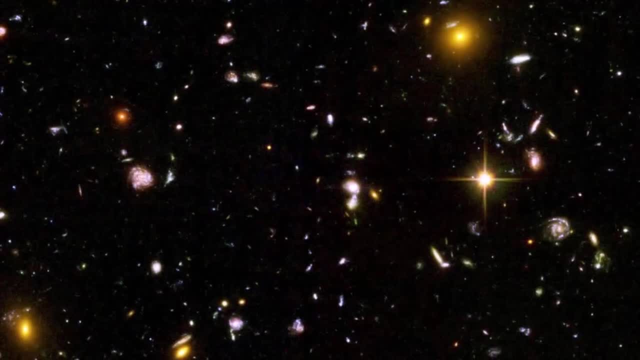 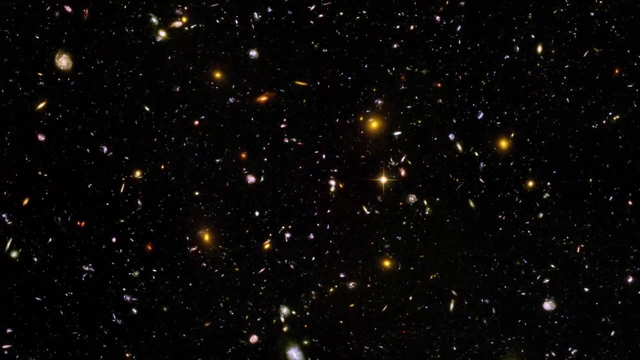 dimensions called p-brains, where p can be any whole number less than 10.. So strings are just one part of the theory, not the whole thing. These other ingredients were hidden because the math used by researchers was not precise enough to reveal them, But with new approaches provided. 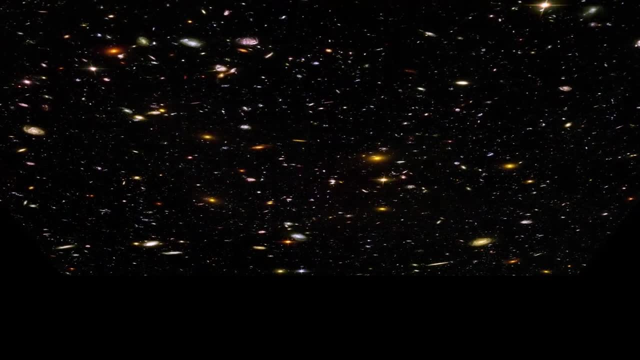 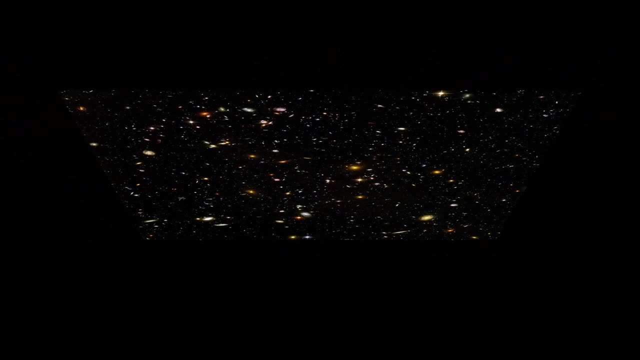 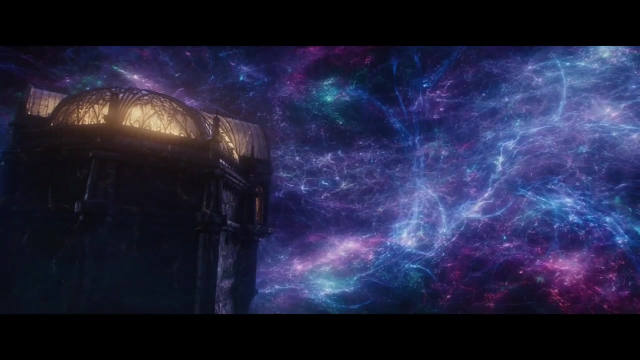 by the M-theory framework, scientists found these higher-dimensional ingredients. The discovery of these extra ingredients doesn't make earlier work obsolete. It just means that there's more to the theory than we originally thought. Depending on their mass, these higher-dimensional objects can: 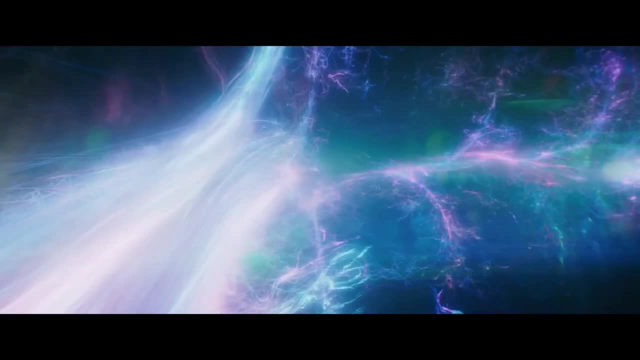 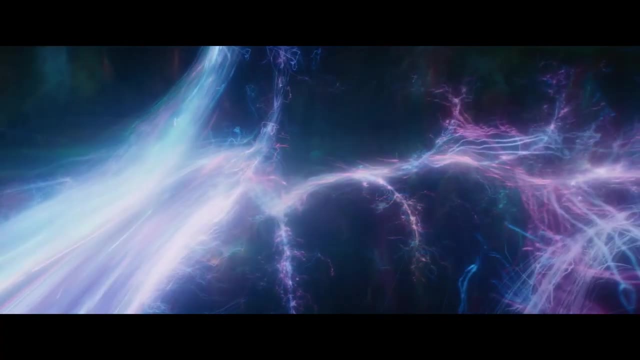 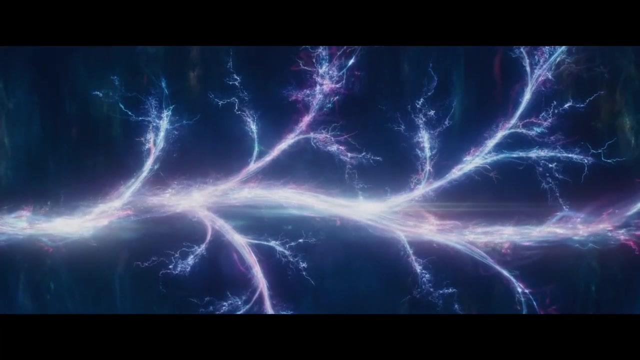 have a significant impact on the physics of string theory. For example, they can wrap around parts of space and affect how it behaves. This idea also leads to the possibility that our entire universe might be like a huge membrane or brain, which is a fascinating idea. 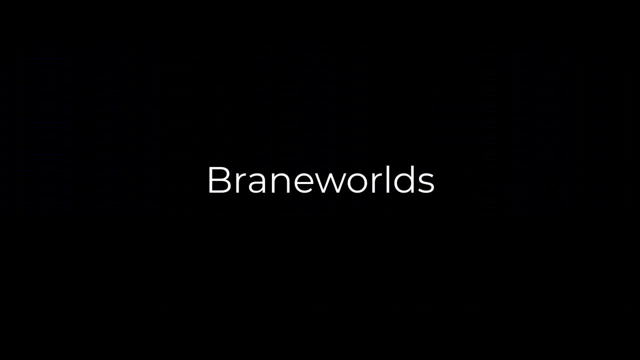 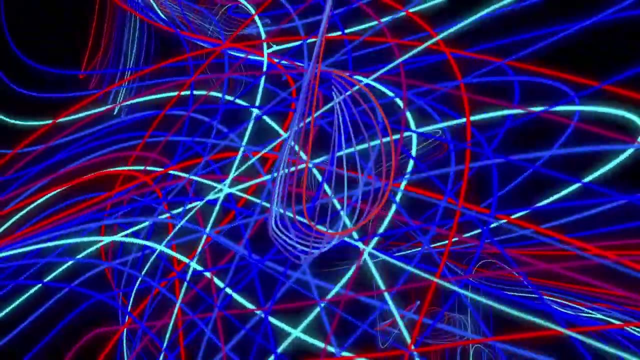 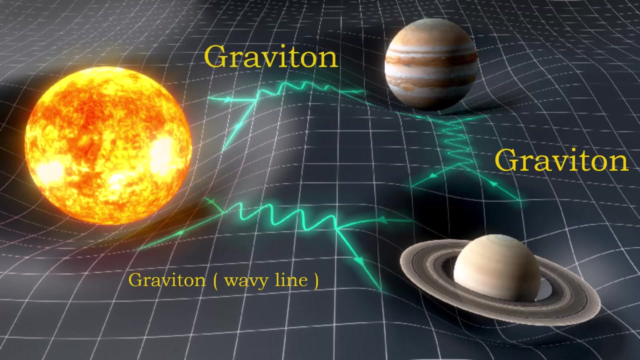 Testing string theory is tricky because strings are incredibly tiny To understand their size. think about the messenger of gravity, the graviton. It's one of the lowest energy patterns that a string can vibrate in, and the strength of gravity is connected to the length of the string. 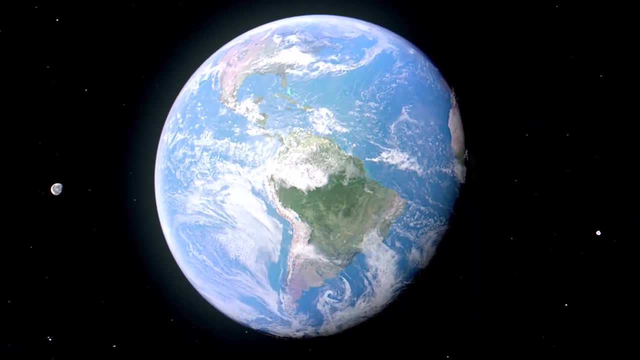 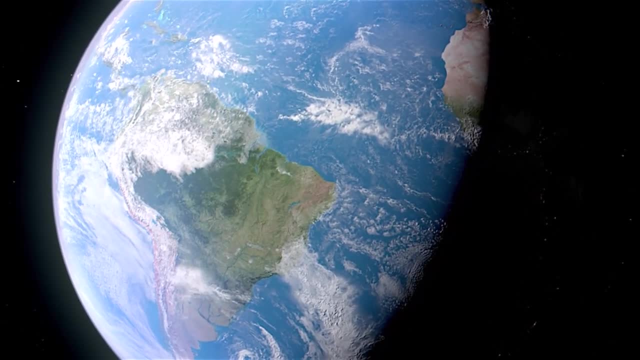 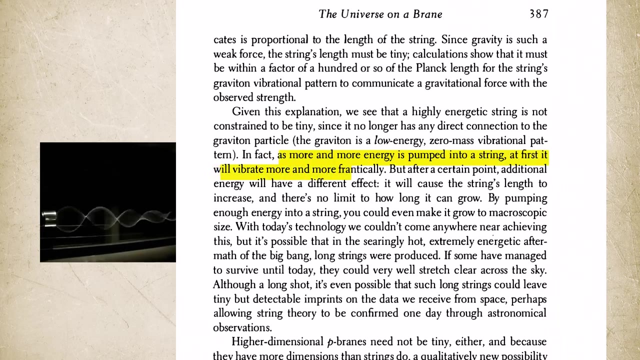 It's about a hundred times the size of the plank length for gravity to work. as we observe it, If you pump a lot of energy into a string, it can vibrate more vigorously, but eventually it will start growing in length. There's no limit to how long it can become, So theoretically, 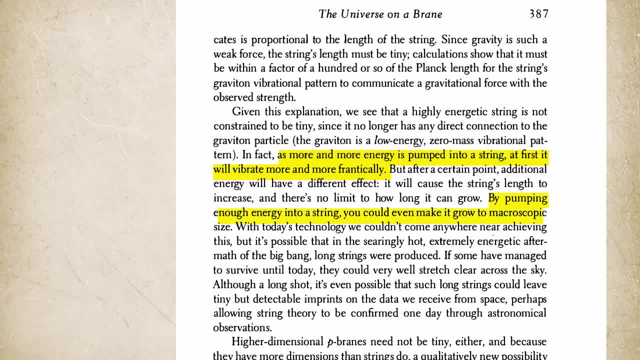 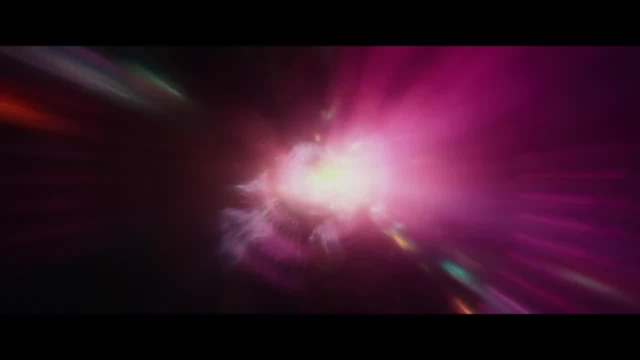 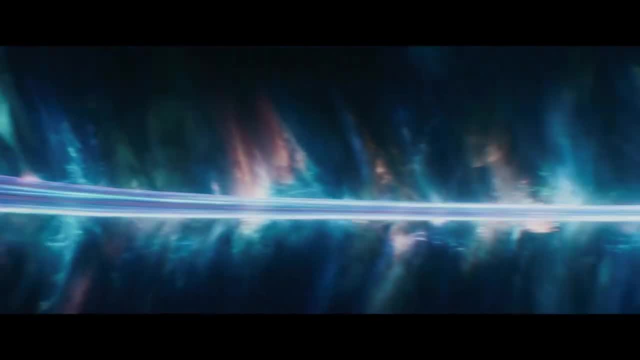 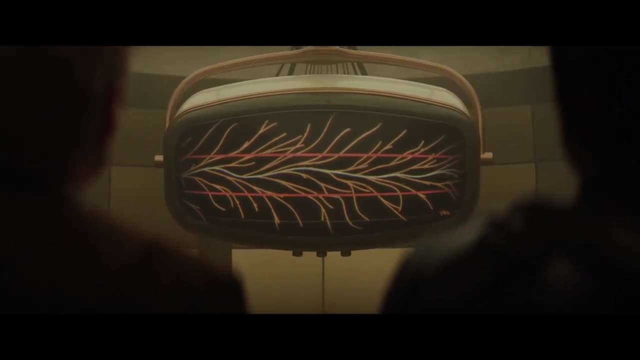 with a ton of energy you could make a string grow to a macroscopic size. With our current technology this isn't possible, But in the incredibly energetic conditions right after the Big Bang, long strings can grow to a macroscopic size. Now there are higher-dimensional objects called P-brains in string theory. 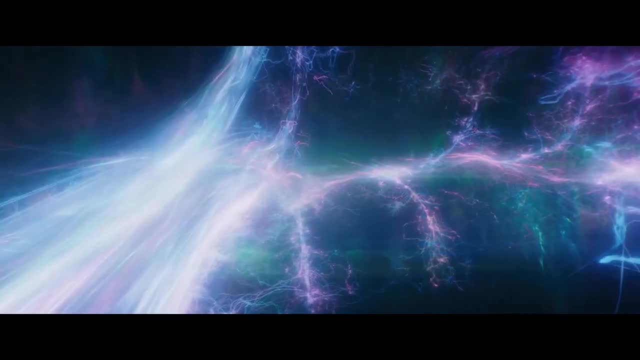 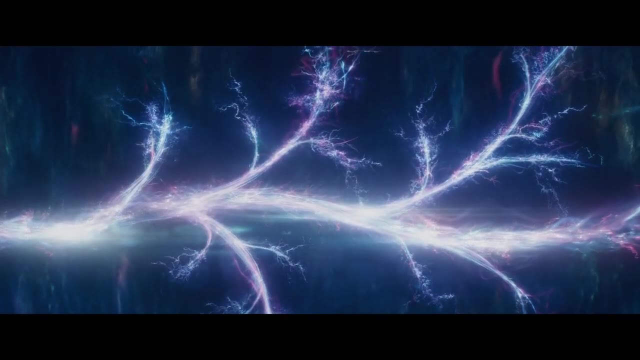 and they don't have to be tiny either, Because they have more dimensions than strings. they offer new possibilities. For example, a long string is like a long one-dimensional object in our three-dimensional world, But a two-brain which has two dimensions is like an incredibly. 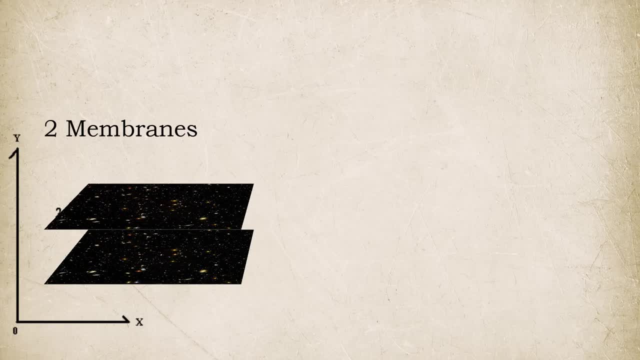 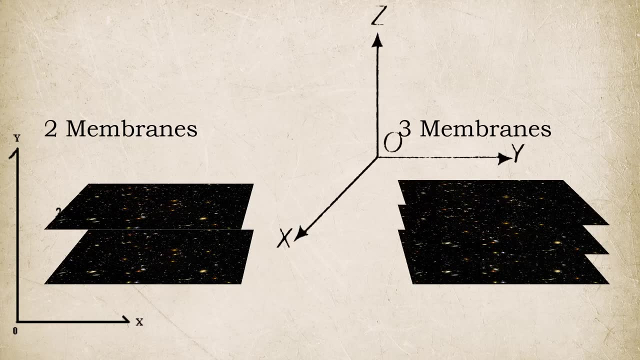 thin but huge surface in our three-dimensional space. A three-brain having three dimensions would fill all the space we know. This leads to a fascinating idea: What if we are living within a three-brain right now? Imagine our world as a three-dimensional. 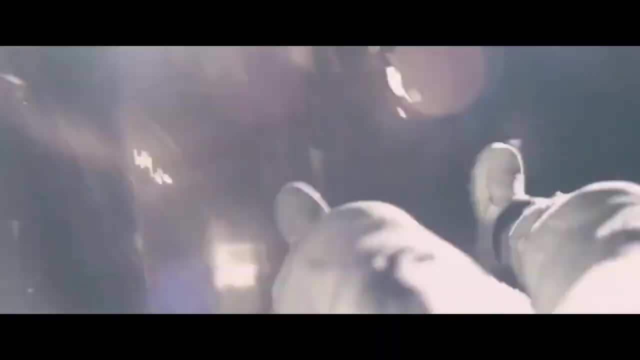 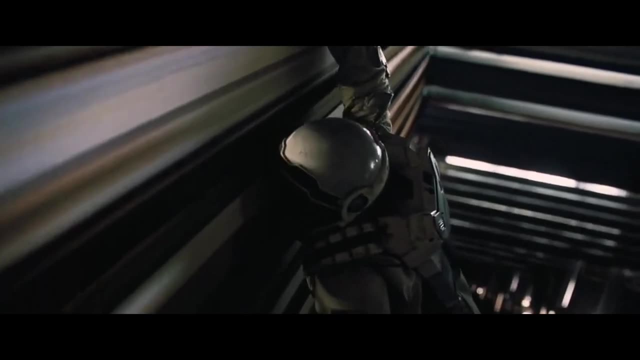 screen inside a higher-dimensional universe of string theory. This idea challenges our understanding of space and time. Could it be that what we call three-dimensional space is a specific three-dimensional space? Could it be that we live within a three-dimensional space? Could it be that? 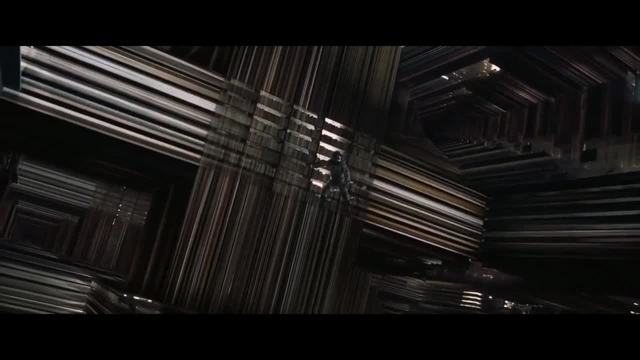 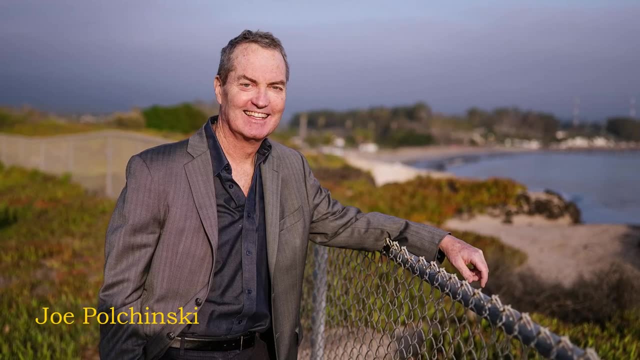 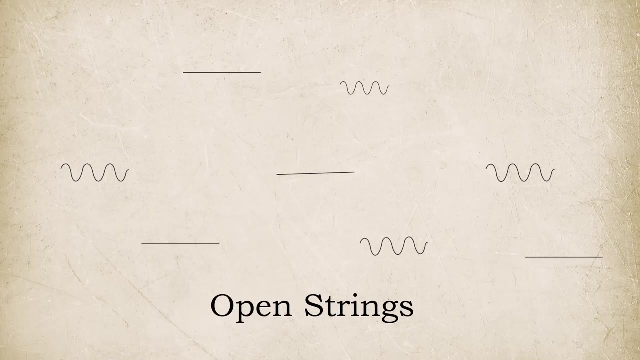 entity. in string theory This possibility called the brain-world scenario. In 1995, after Witten's groundbreaking discovery, Joe Polchinski revisited an intriguing aspect of string theory. He found that open strings which have two loose ends could be restricted to move. 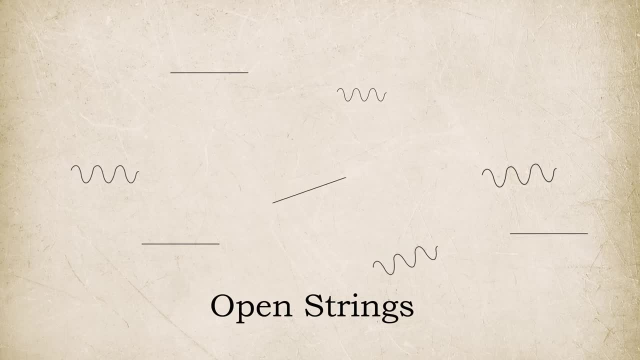 in specific shapes in space. These shapes could be one-dimensional, two-dimensional or even higher-dimensional. One big question was: what are these open strings stuck to? Unlike real-world objects like wires or pinball tables, these regions of space seem to be just. 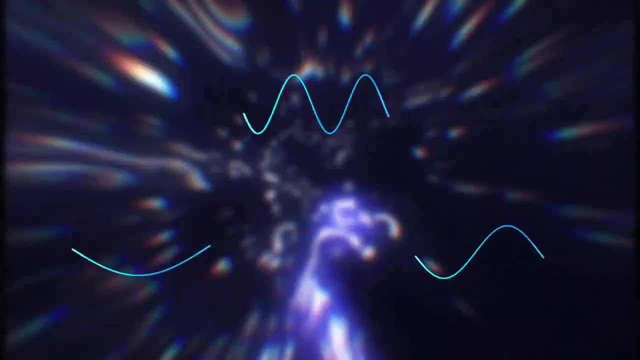 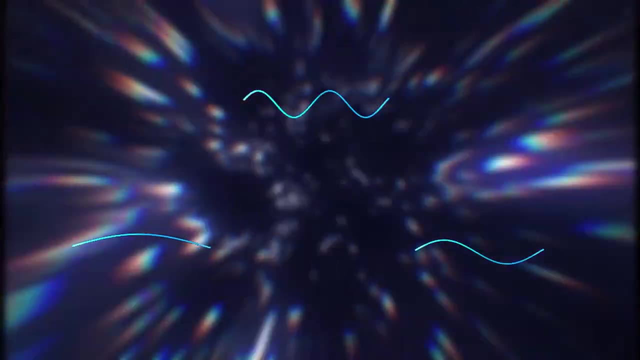 that regions of space. There wasn't an obvious answer until the advent of M-theory. M-theory revealed that these regions are occupied by P-brains, which are higher-dimensional objects. They grip the endpoints of open strings limiting their movement within the P-dimensional. 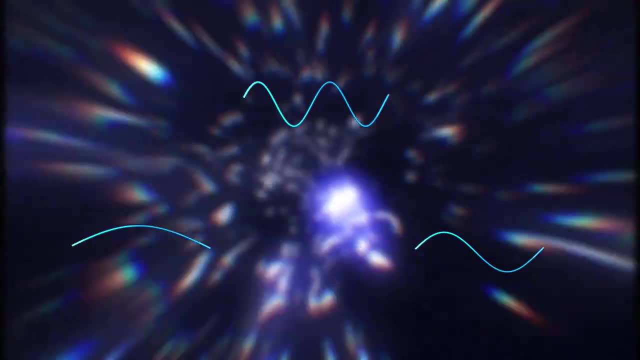 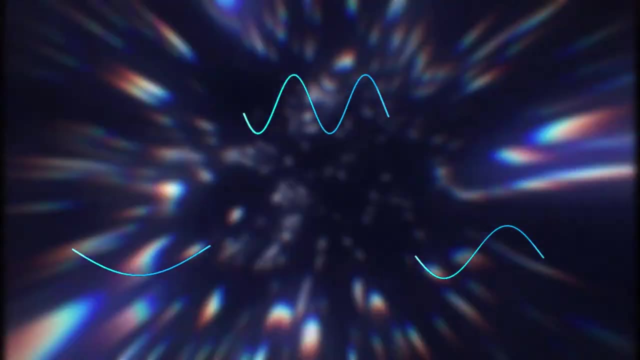 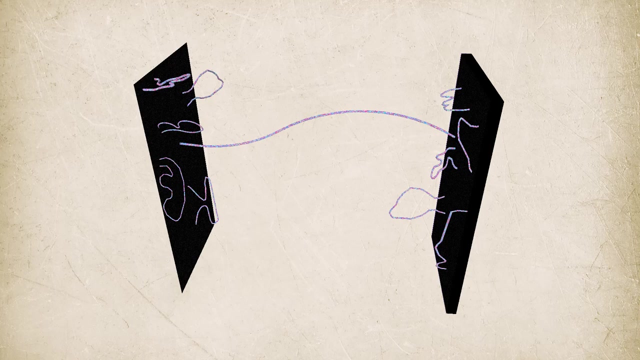 space they occupy. Think of it this way: If you have two-dimensional brains, open strings can move freely on and within them, but can't leave the brain. Brains are like cosmic Velcro. when it comes to open strings, they stick to them. You can even have one end of an open string. 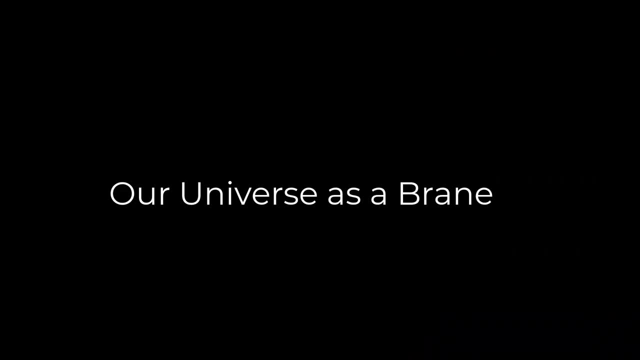 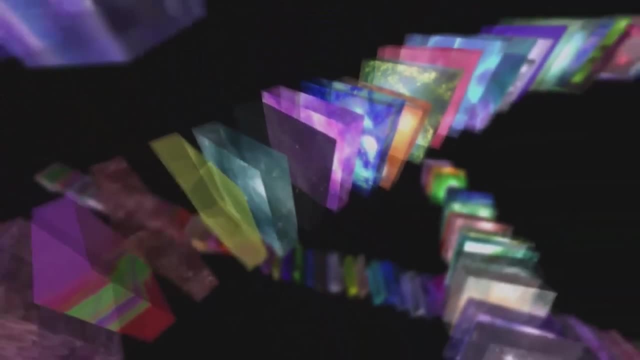 stuck to one brain and the other end to a different brain. Imagine if our universe is like a giant three-dimensional screen and our four-dimensional screen again, any two-dimensional for you, and the space of wisdom giving you the second dimension. In this way, you 물� won't just. 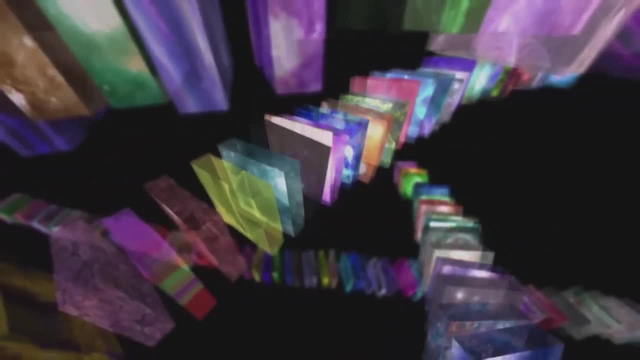 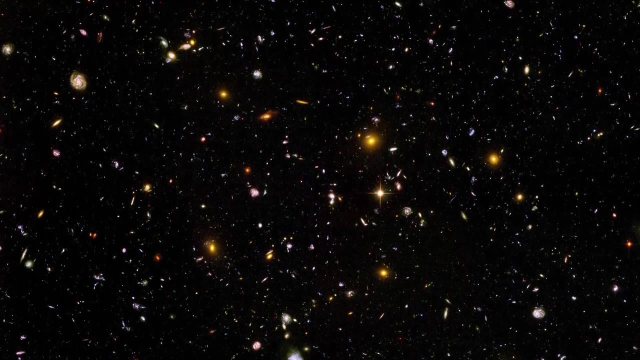 happen and get stuck in the same space. You're in picture and yourself You're not going to be no-knowers. spacetime is like a movie playing on that screen. In this scenario, our familiar spacetime isn't just an abstract concept. It's a real, physical thing, A three-brain. Now you might wonder why. 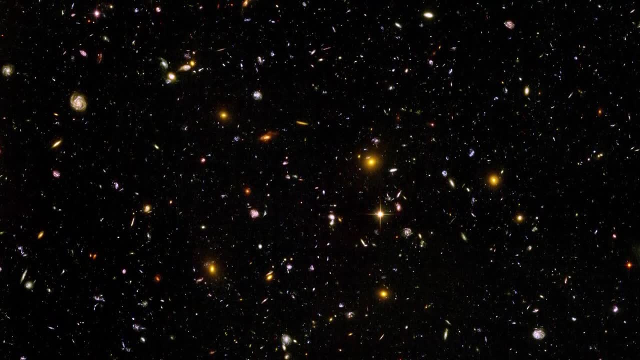 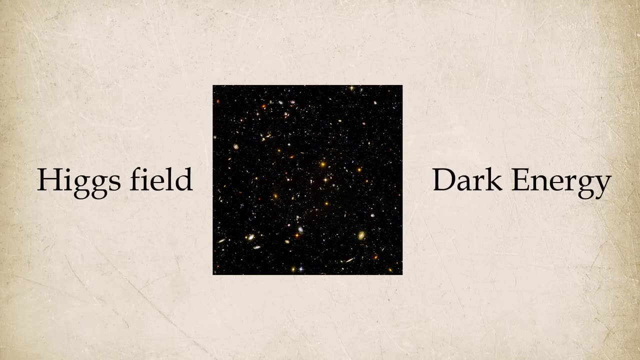 we can't see or feel this three-brain, if we're supposedly living within it. To explain this, think about other invisible things in our universe, like the Higgs field or dark energy. These things don't directly show themselves to us, but we can still detect their effects. 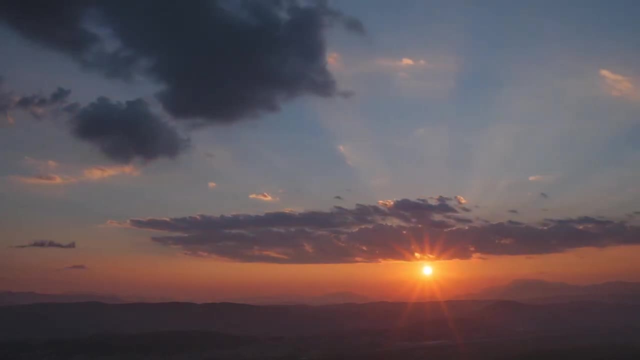 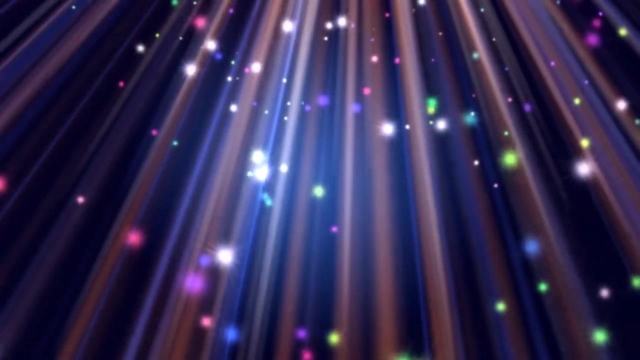 When it comes to the three-brain, things work a bit differently. It turns out that only certain types of vibrations in this theory produce particles of light or photons. These photons can move freely within our three-brain, but can't leave it. This makes the three-brain seem. 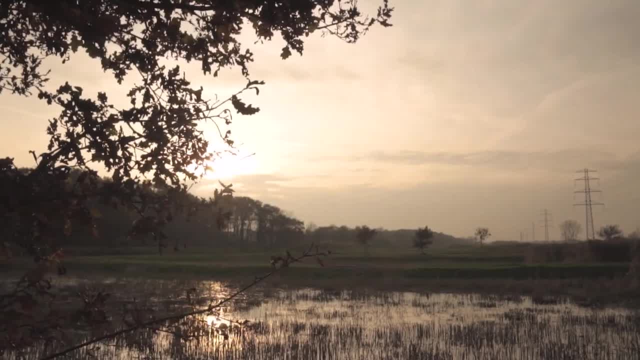 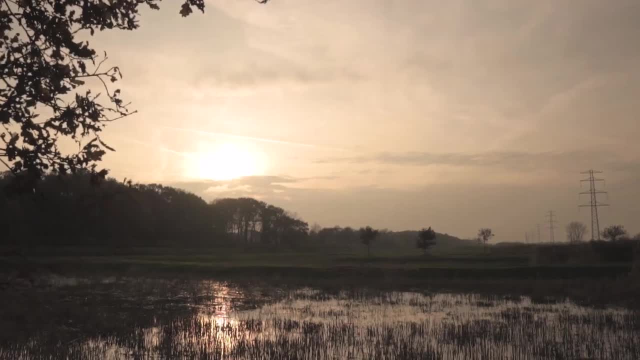 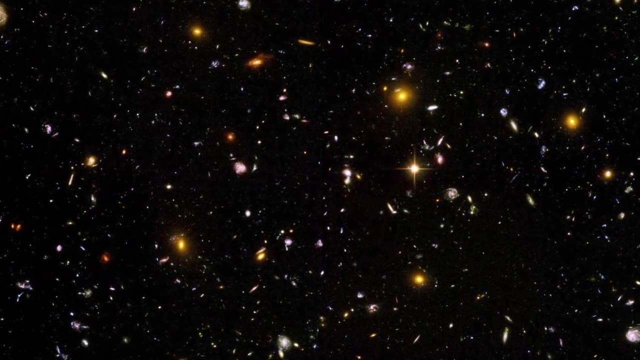 completely transparent and invisible to us. Similarly, other forces and particles we know, like the electromagnetic force and particles of matter, are also stuck within our three-dimensional dimensions. They can't explore or detect the extra dimensions of M-theory. Now here's where. 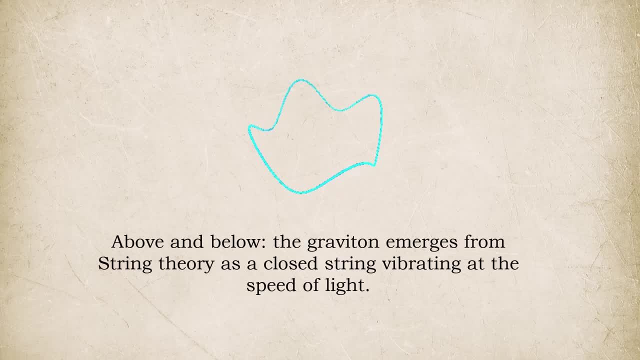 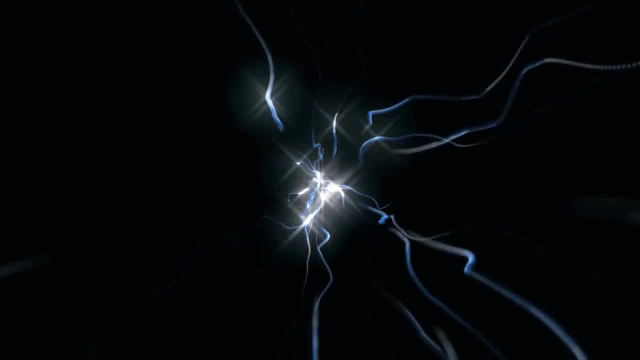 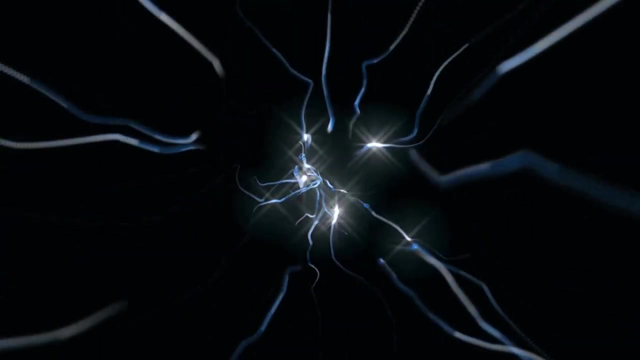 it gets interesting. The gravitational force is special. It's carried by particles called gravitons, which come from a different type of vibration. in M-theory, Unlike the other forces, gravitons can escape our three-brain and interact with the extra dimensions. So while most forces, 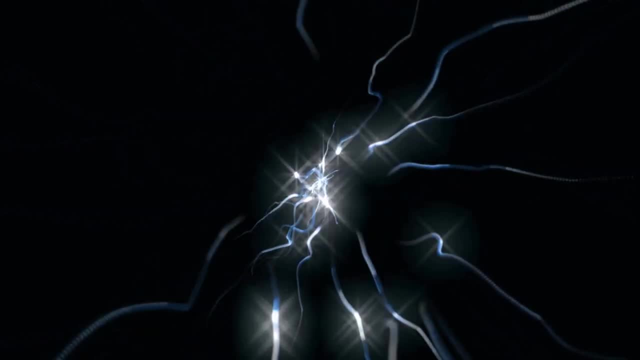 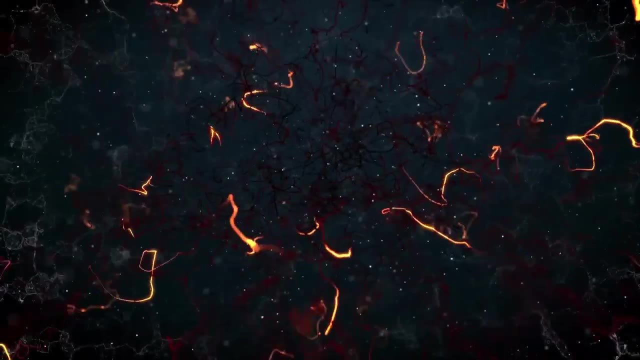 and particles are confined to our three dimensions. gravity can reach beyond. This means that gravity is our only way to connect with the extra dimensions. But how big could these extra dimensions be before we'd notice them through gravity? That's a critical question. 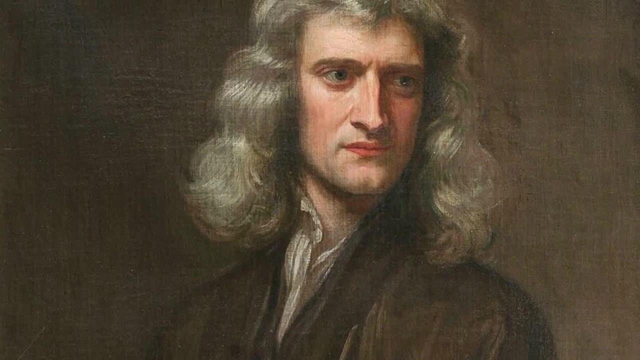 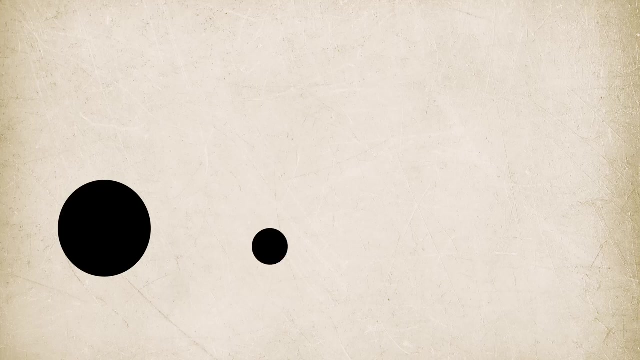 and we'll explore it next. Back in 1687, Sir Isaac Newton came up with a law about how gravity works. He said that the force of gravity between two things gets weaker when they move apart. Newton used math to explain exactly how this force gets weaker. He called it the 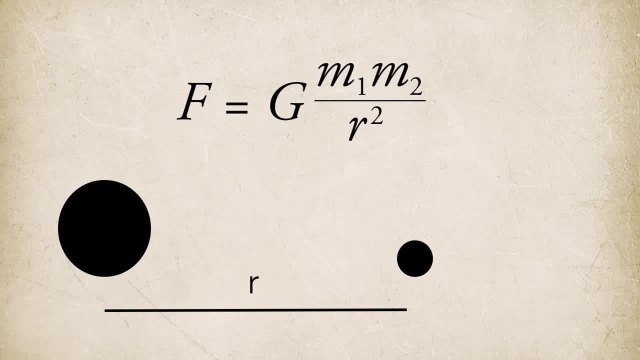 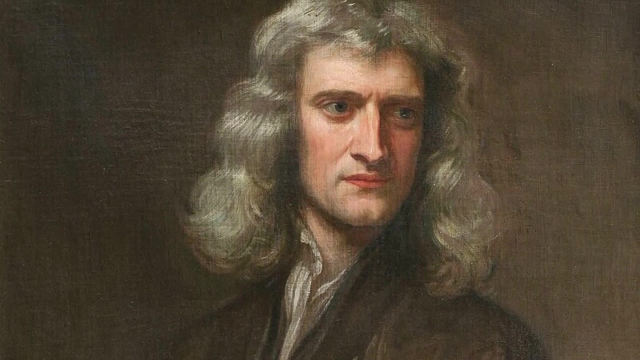 inverse square law, which means that if you double the distance between two things, the gravity force between them becomes four times weaker, and if you triple the distance, it becomes nine times weaker, and so on. This law has been proven correct for hundreds of years. Now you might. 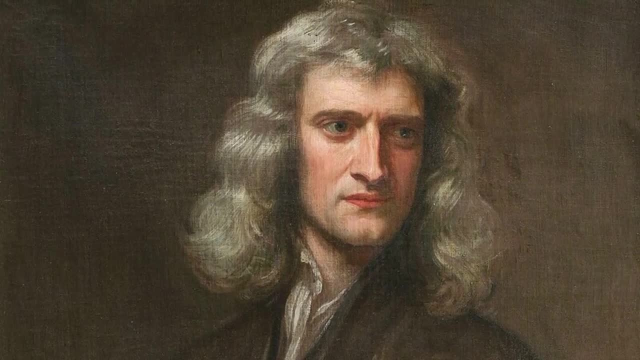 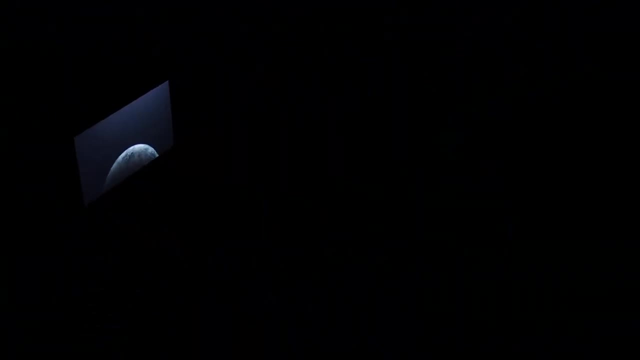 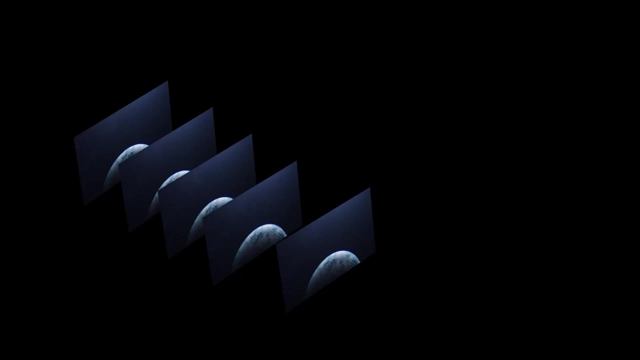 wonder why gravity follows this specific rule and not some other way. Well, the answer has to do with how many dimensions our space has. Imagine space as a screen and objects in it as dots on that screen, If our universe had two or even just one dimension, instead of three. the law of gravity. 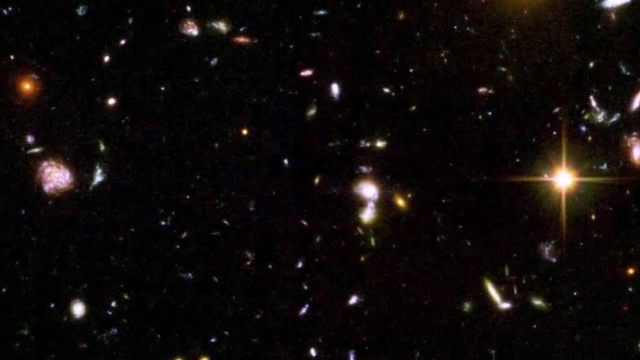 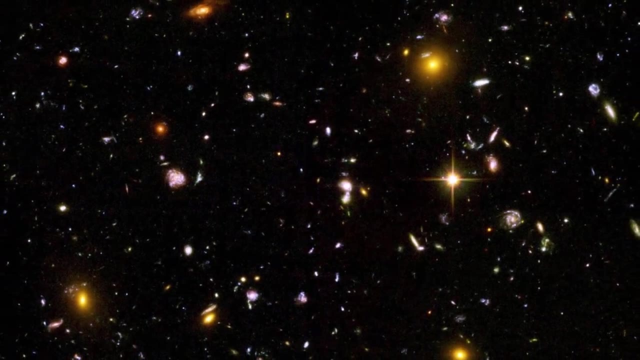 would work differently. In a two-dimensional universe, gravity would drop in proportion to separation. In a one-dimensional universe, gravity wouldn't drop at all with separation. It would stay constant. So you might think that, because gravity follows the inverse sequence, gravity follows the inverse sequence, But that's not the case. Gravity follows the. 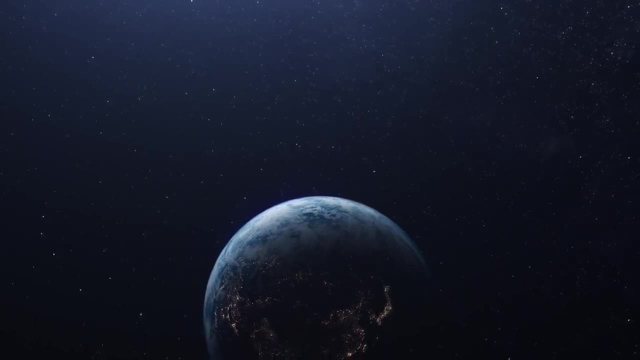 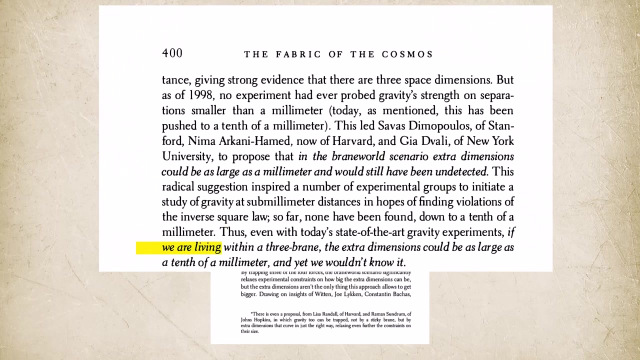 inverse sequence. Gravity follows the inverse sequence. Gravity follows the inverse sequence: Square law: in our universe we must have three dimensions, But we've only tested this law down to very tiny distances, about a tenth of a millimeter. If our universe had extra hidden? 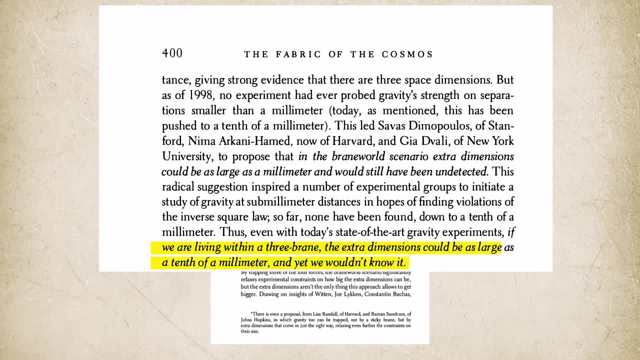 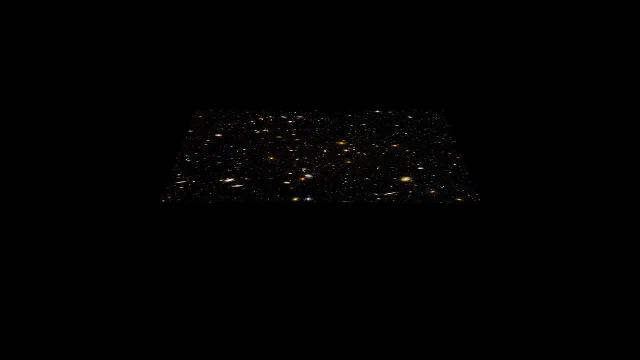 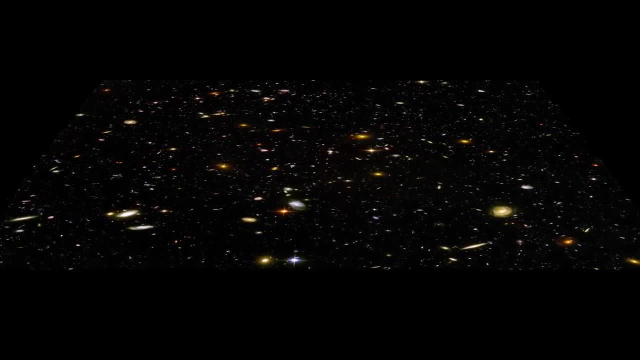 dimensions. we wouldn't have noticed them with our experiments so far. Imagine living in a two-dimensional universe but not knowing it, because our tests only work down to a certain scale. When objects are very close, you'd see gravity following the 2D rule, But when they're, 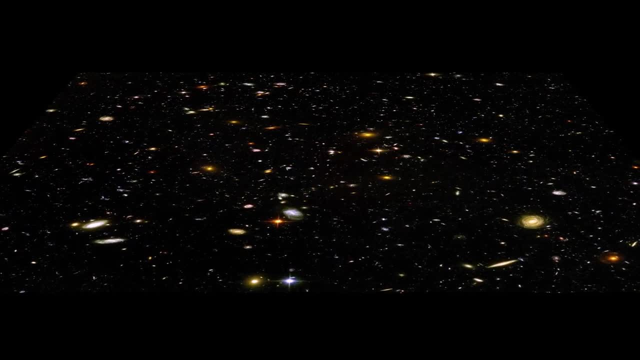 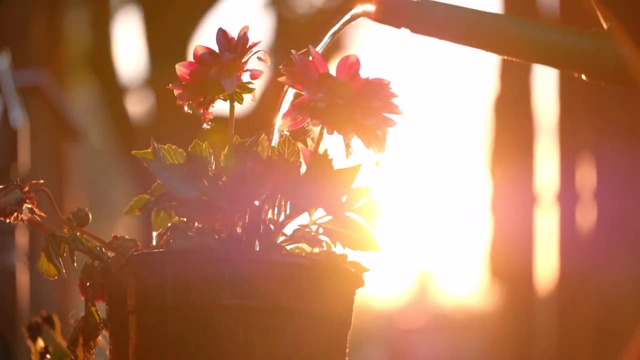 farther apart, it would seem as if the gravity force stays constant as we've known it for centuries. In our real three-dimensional universe, we've never tested gravity at scales smaller than a millimeter. This leaves room for the possibility that there could be extra dimensions as large as 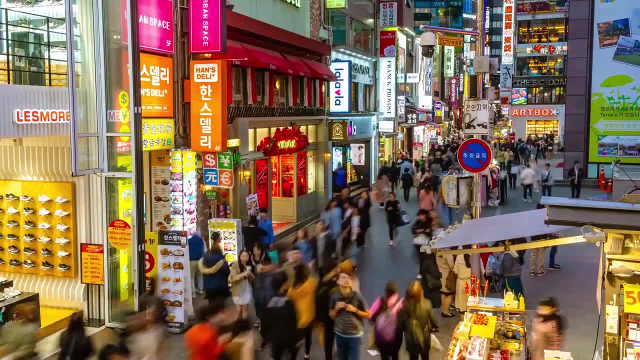 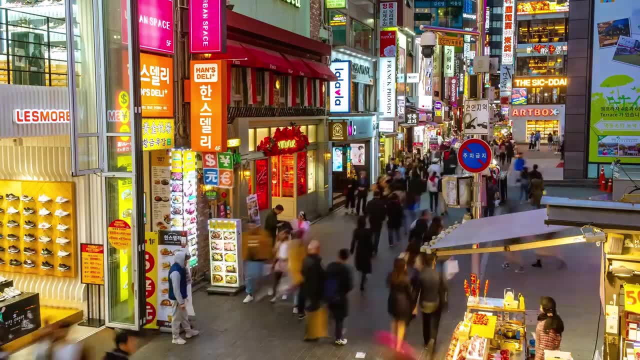 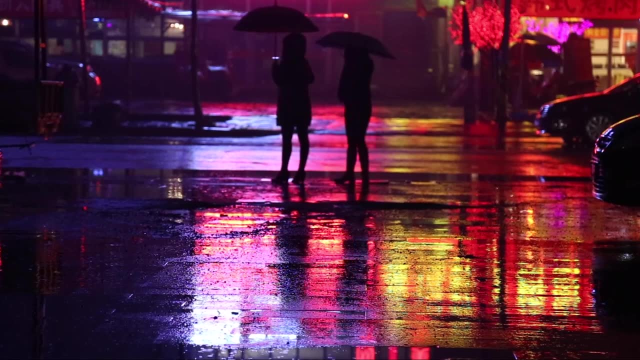 a millimeter, and we wouldn't have detected them yet. This idea led scientists to conduct experiments looking for deviations from the inverse square law at very small scales, but so far they haven't found any. This means that even if we live in a three-brain scenario with hidden dimensions, 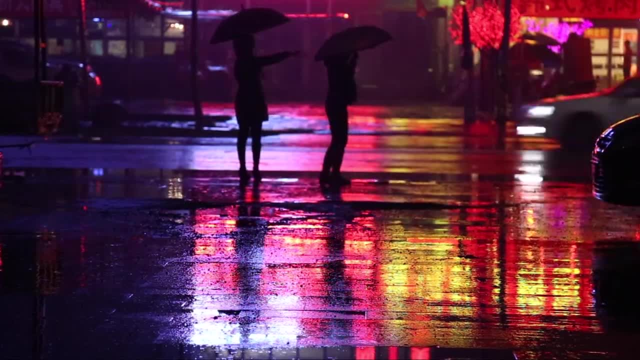 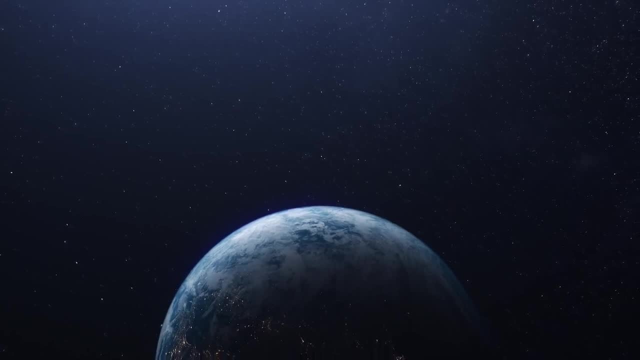 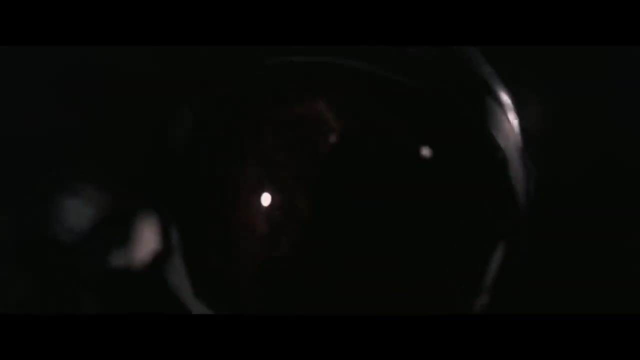 they could be as big as a tenth of a millimeter, and we wouldn't know it. It's a remarkable realization that our most advanced instruments might still miss some hidden aspects of the universe. The idea that we might live in a large three-brain is just a possibility, and so is the 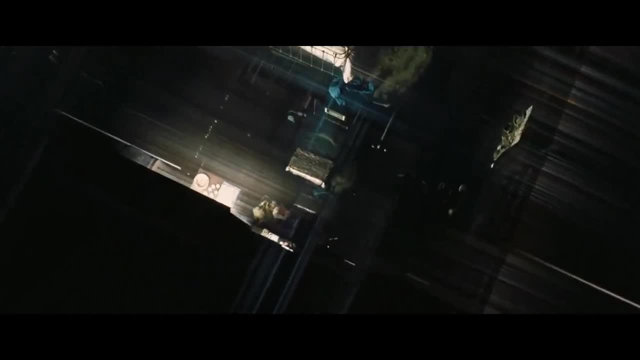 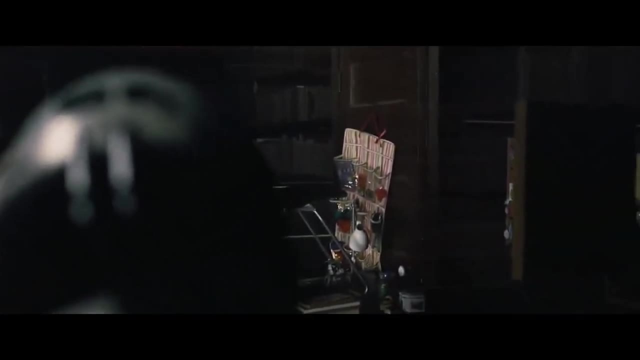 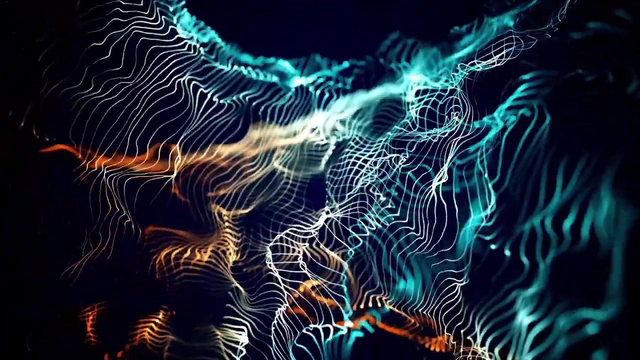 idea that the extra dimensions and strings could be much bigger than we thought. These possibilities are exciting because they could turn string theory into an experimental science, But we don't know for sure if these possibilities are likely or not. It's hard to predict If the strings are larger. 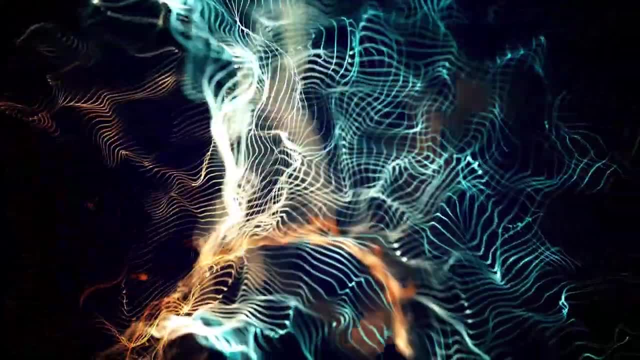 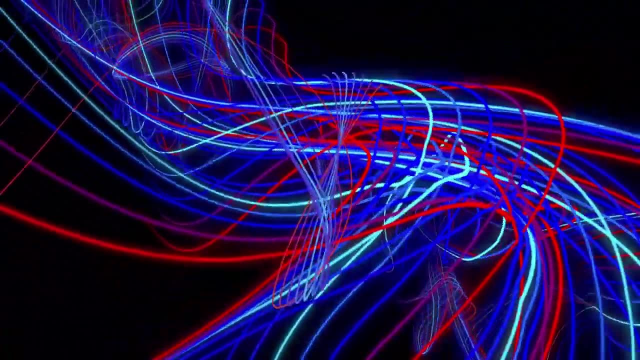 or if some of the extra dimensions are larger, it would have a big impact on upcoming experiments. For example, if strings are as big as 10 to the power minus 18 meters, the particles produced in high-energy collisions could have masses that are within reach of the Large Hadron Collider. 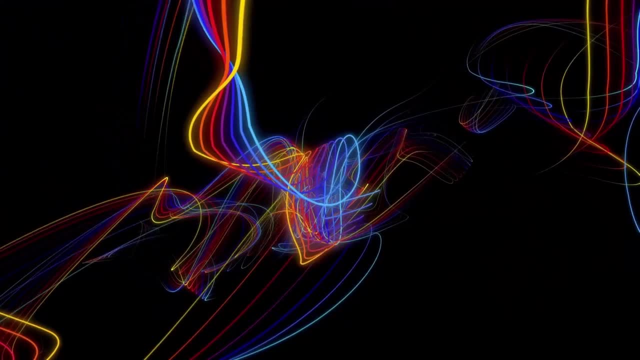 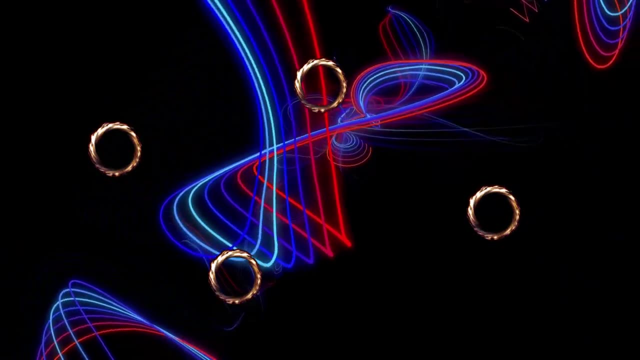 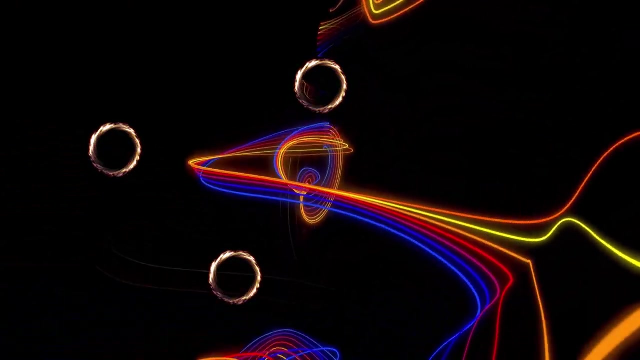 This could lead to the creation of many new particles and it would be a clear sign of string theory in action. Additionally, in the brain-world scenario, these high-energy collisions might even create miniature black holes. These tiny black holes wouldn't be a threat and would disappear. 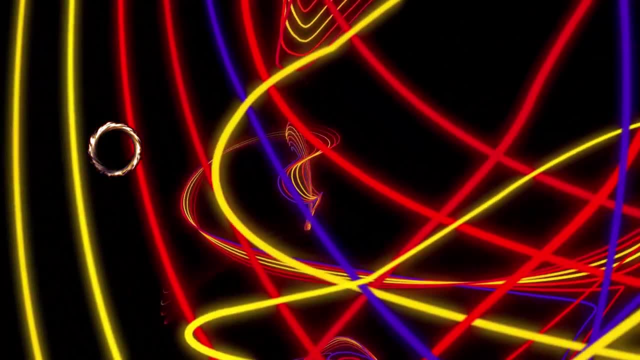 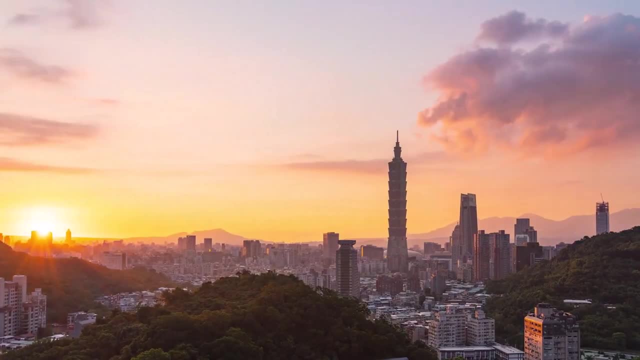 quickly, but their creation would provide strong evidence for some very unusual ideas in physics. In our everyday experience, we encounter two types of particles. One is the black hole and the other is the string. The black hole is made up of a variety of things related to time. Some have clear beginnings and ends. 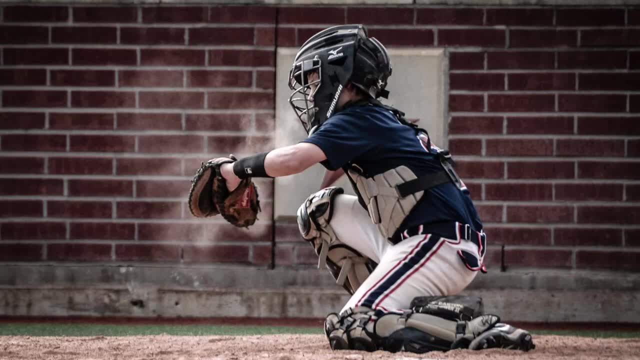 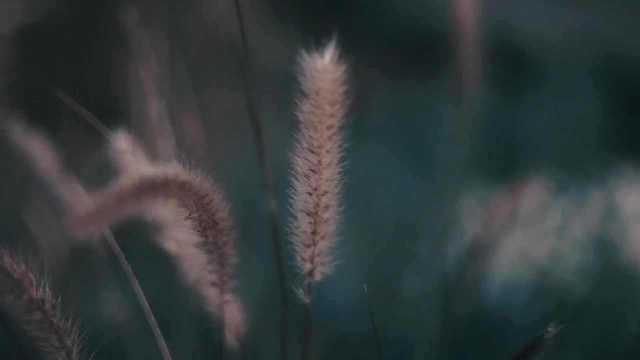 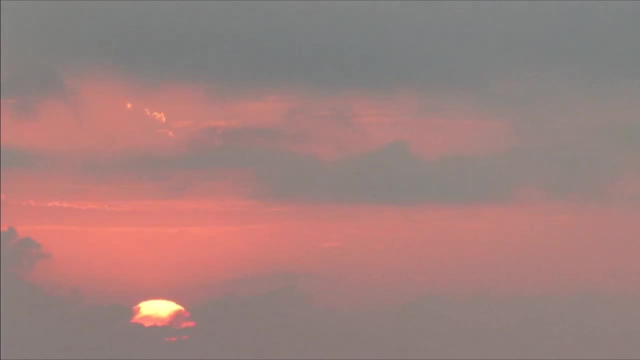 like books, baseball games or human lives. Others repeat in cycles, like the changing seasons or the daily sunrise and sunset. Even though cyclic things seem to keep going forever, they also have beginnings and endings. when we look closely, For example, the sun has been rising and setting. 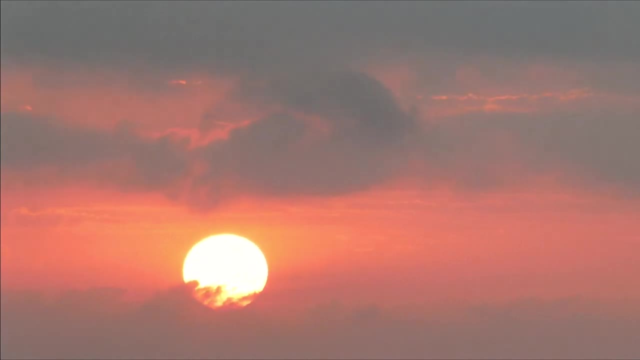 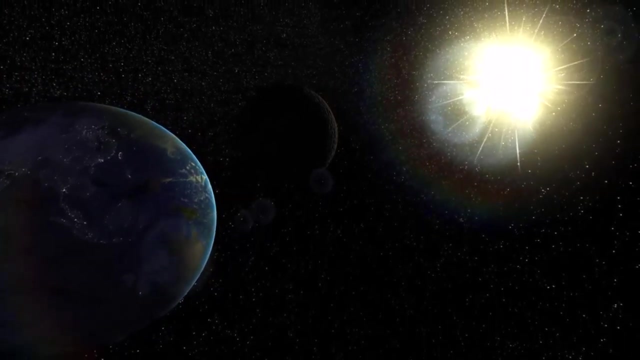 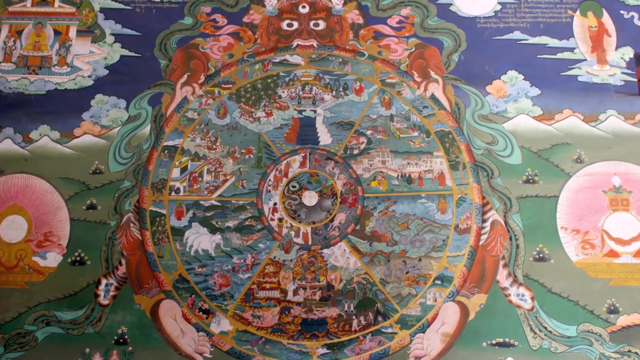 for about 5 billion years, but before that it didn't exist. and in another 5 billion years it will become a red giant and engulf planets like Earth, so there won't be any more daily sunrises and sunsets. Ancient cosmologies often thought of the world as an eternal cycle. 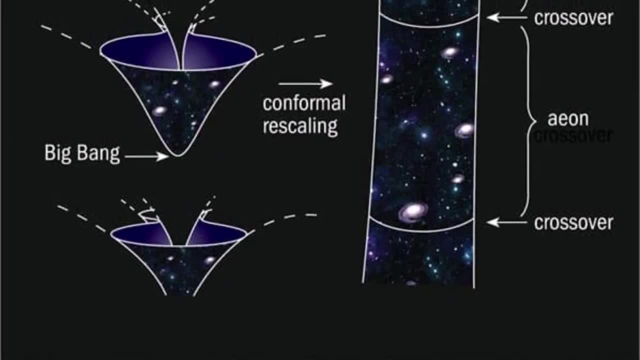 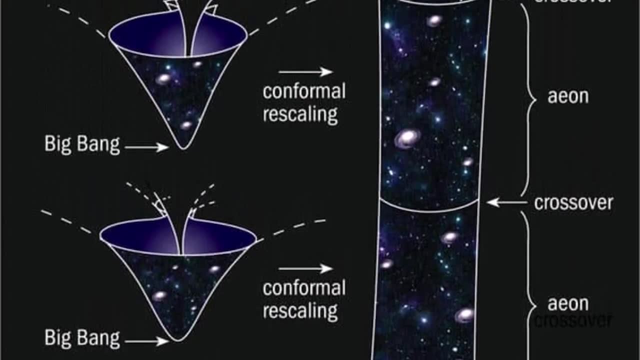 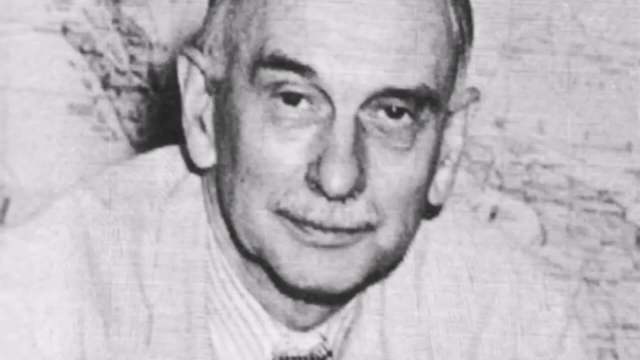 with no real beginning or end. Cyclic cosmological models were proposed to explain how the universe might work, and one famous idea suggested that the universe expands, then contracts and then bounces back to expand again in a never-ending cycle. This concept was introduced by Richard Tolman in the 1930s. Tolman's idea relied on a spherical 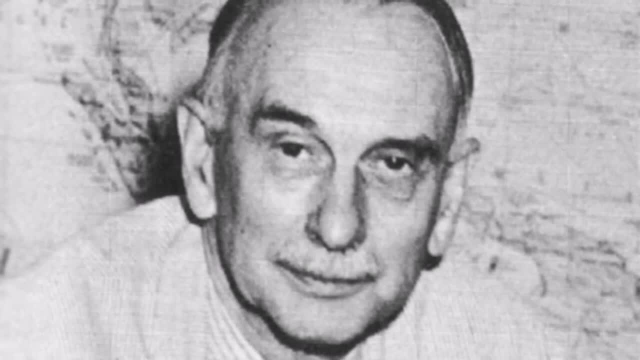 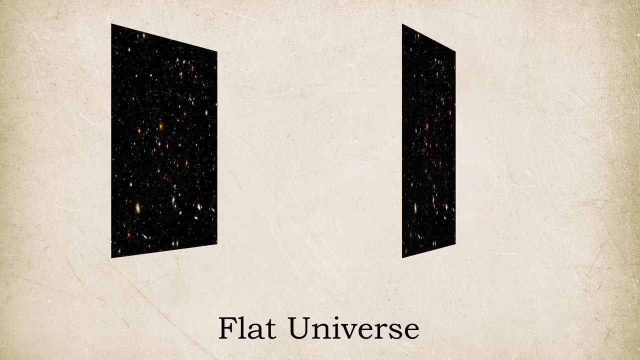 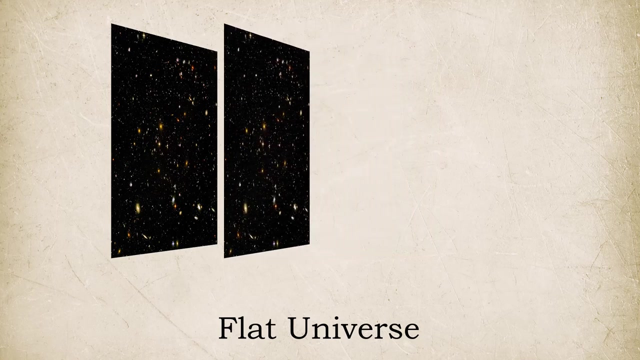 universe, but this was later disproven by observations. A new version of cyclic cosmology has been developed, using string theory, which involves a flat universe. This new model, proposed by Paul Steinhardt and Neil Turok, suggests that our universe is like a three-dimensional. 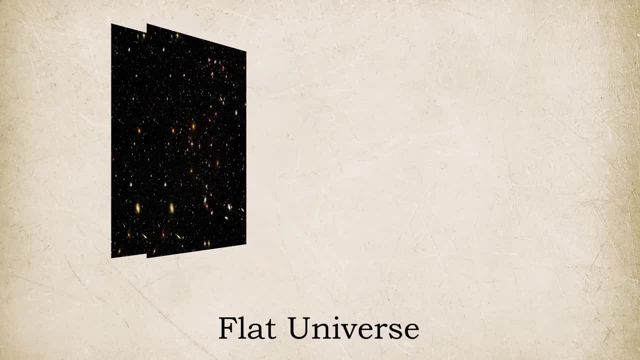 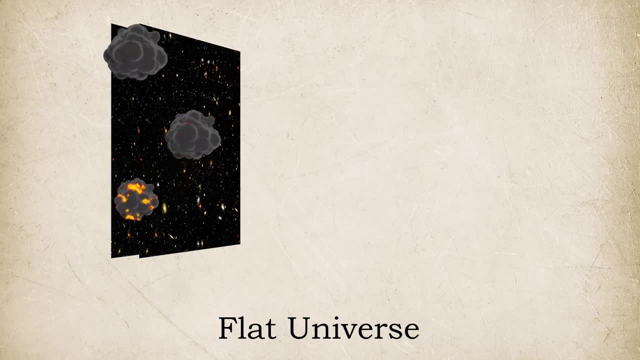 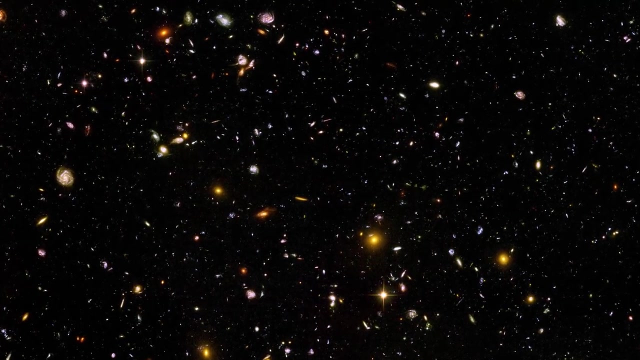 sheet and it collides with another similar sheet every few trillion years. This collision acts like a bang and starts a new cycle of cosmic evolution In this model. during each cycle, the universe expands, cools down, forms, stars and galaxies. 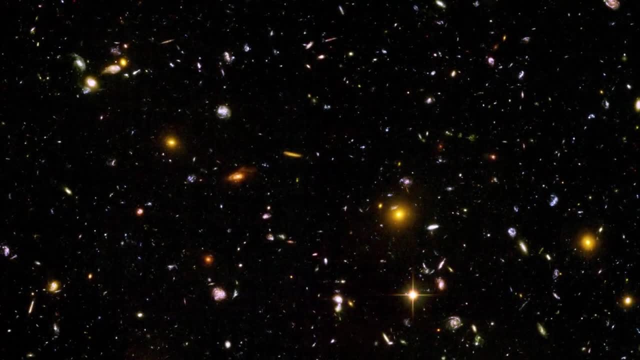 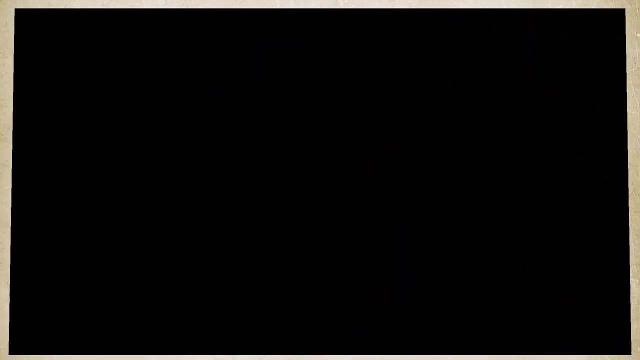 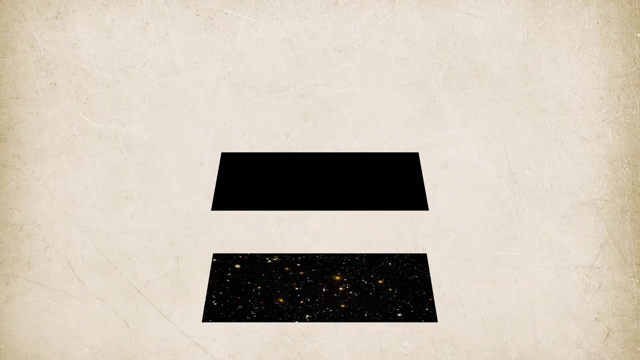 and eventually experiences an accelerated expansion phase driven by dark energy, similar to what we observe today. After trillions of years, the universe becomes almost empty and uniform. Then it approaches the other sheet, Quantum ripples create tiny irregularities and another collision initiates a new cycle. 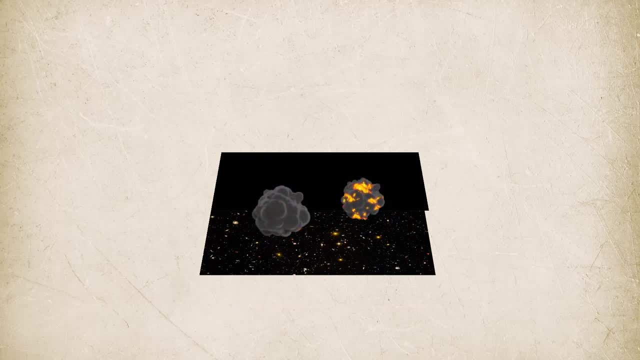 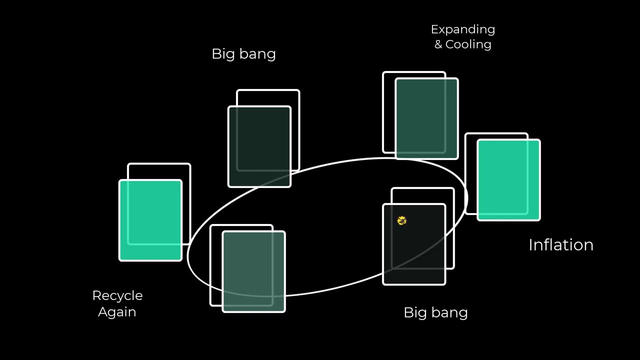 While this cyclic model is different from the widely accepted inflationary theory, they share similarities such as using quantum fluctuations to generate initial irregularities. Additionally, the cyclic model takes its time to resolve cosmological issues, over trillions of years, making the universe flat and uniform before starting a new cycle. 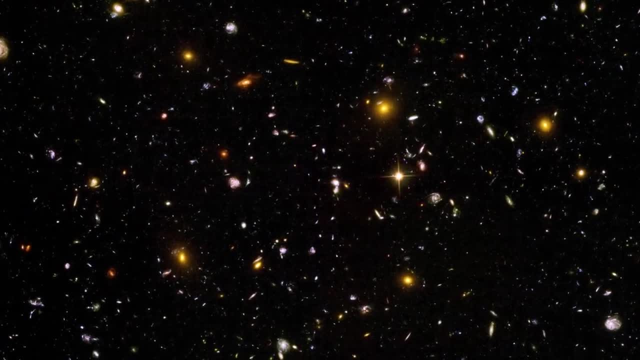 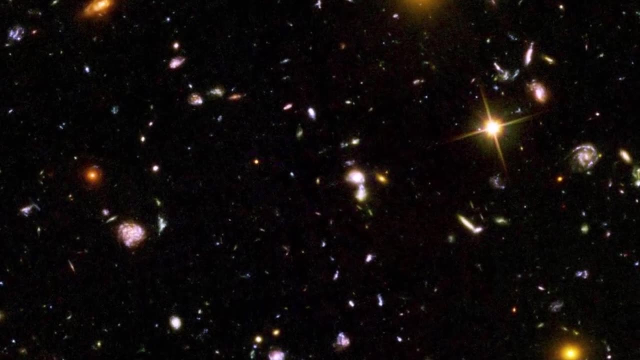 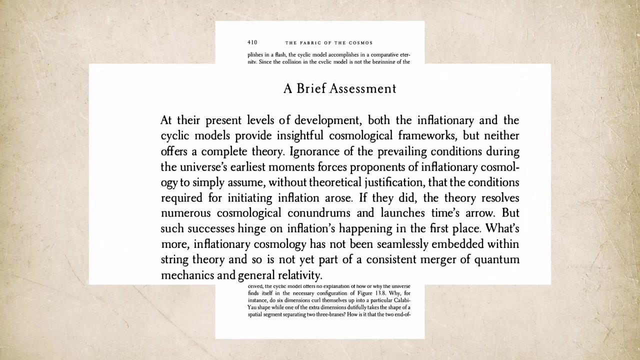 Both the inflationary and cyclic models provide useful ways to think about the universe, but neither is a complete theory yet In the inflationary model, there's a lack of understanding about what conditions were like at the universe's very beginning. It assumes that the right conditions for inflation existed, without a clear explanation of why. 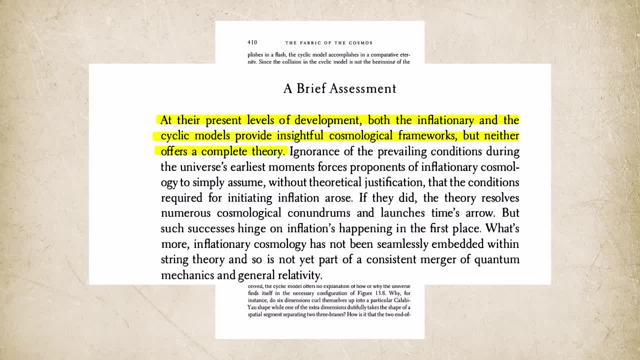 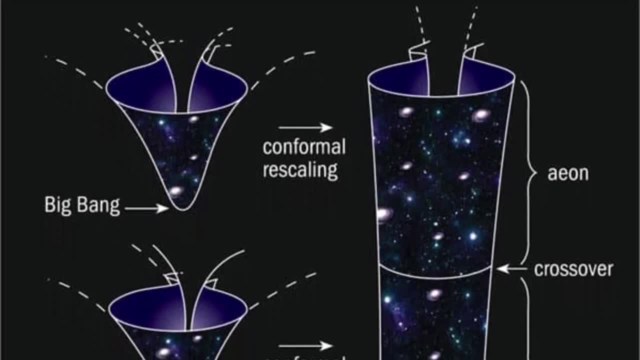 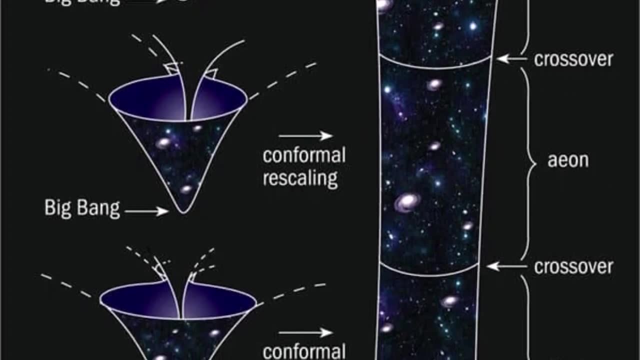 If inflation did occur. it solves many cosmic puzzles, but it hasn't been fully integrated with string theory, The String Theory. The cyclic model also has its issues. It faces questions about how and why the first cycle started and why the universe is, in its specific configuration, The most significant 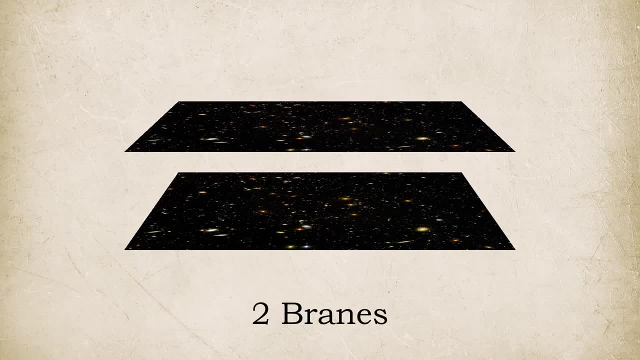 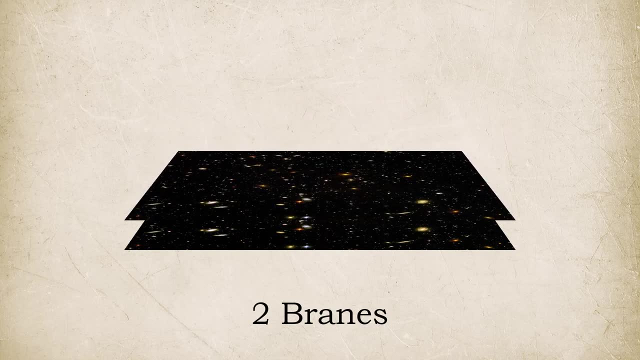 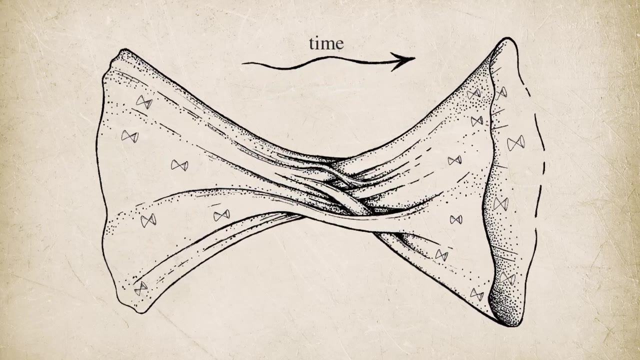 challenge is understanding what happens when the two brains collide in the cyclic model, as the current mathematical equations aren't clear on this point. One positive aspect of the cyclic model is its natural incorporation of dark energy and the observed acceleration of energy. The cyclic model can almost always be in financial. hasn't problems, But ZeplonSum. 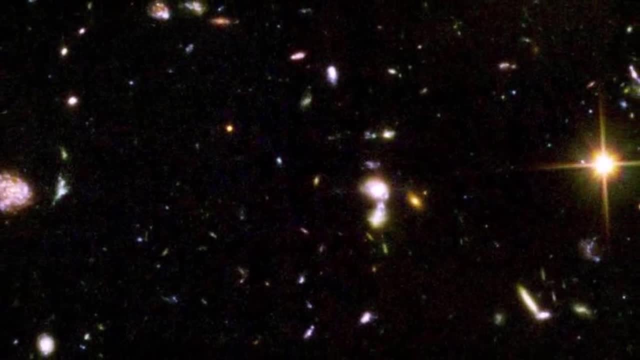 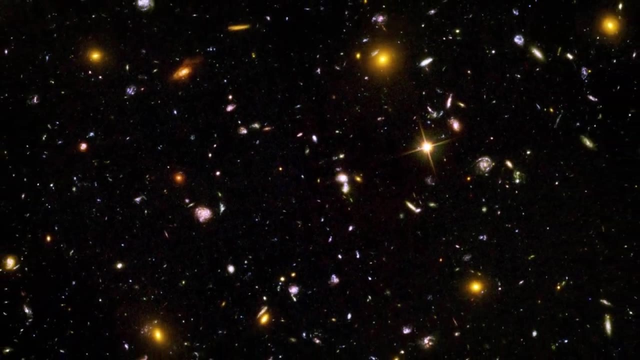 benefits both of these in evaluating the situation, and for which it has thisrando. Starting with a simple guess, The cyclic model gives information for what occurred in the life tonnes given by the trajectories, the patterns of temperature and also the energy yourself've clean and 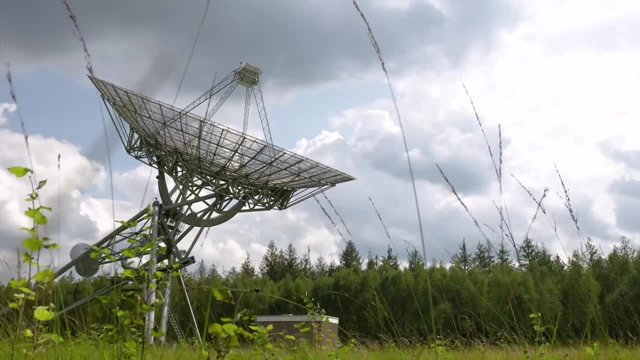 as far as phenomena, let's consider the productiveof your evaluation by comma tranks. Does this have any effect on your own yıl, or the amount you have divided intoites, or the change in ratio, and indeed on your concept of your coffee? This adds up all the 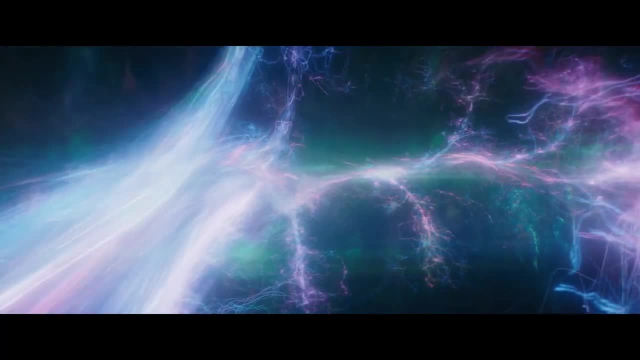 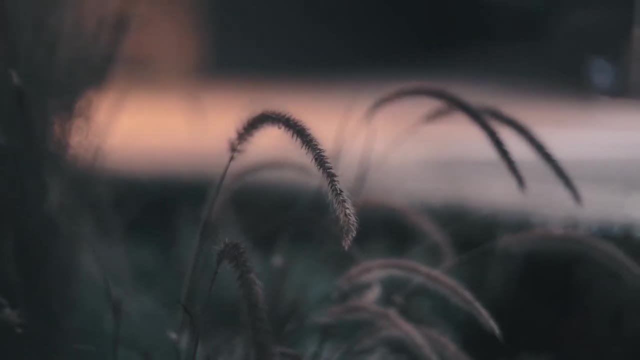 problems that you may have produced. So what's the only real reason to ask this question? in the next slide, Let us find out. cosmological model it inspired are still just ideas without strong confirmation. If we live on a three-brain, it would answer the age-old question of whether three-dimensional space is. 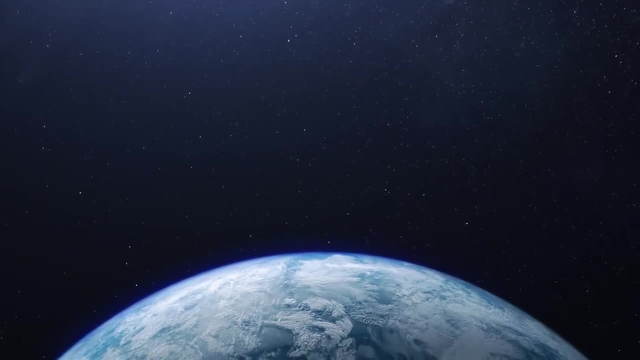 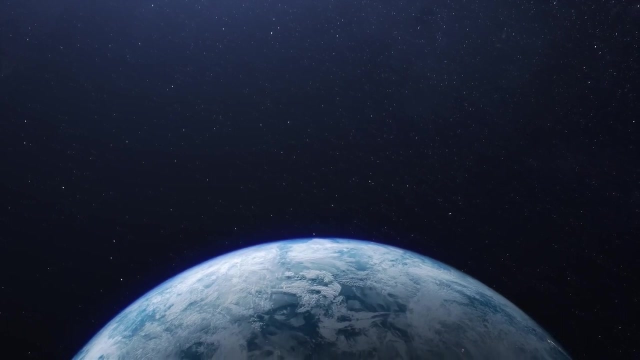 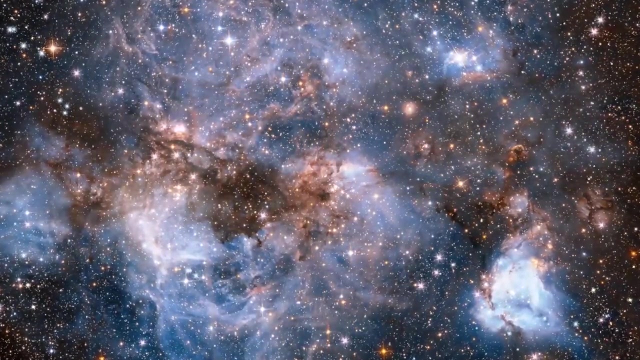 something real. In this case, space would indeed be something tangible. It might not be unique either, as there could be many other brains of different dimensions in the higher-dimensional realm of string theory. If our universe's evolution is driven by collisions with another, 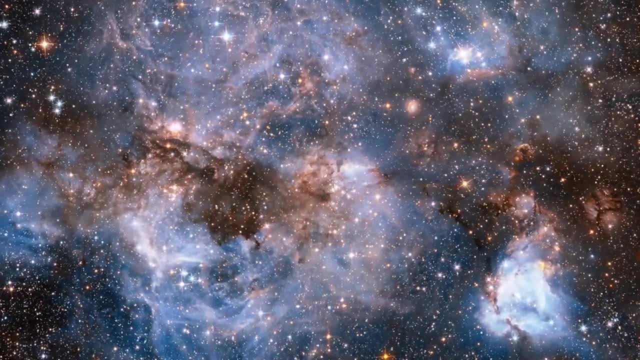 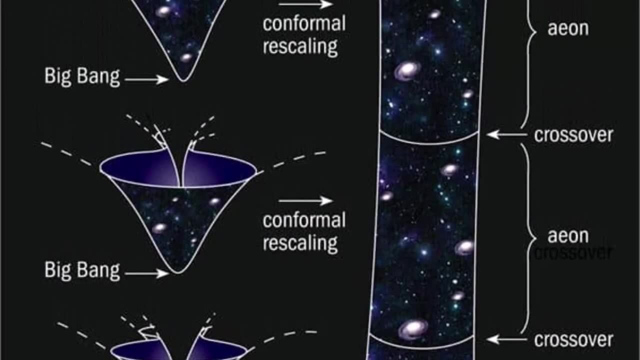 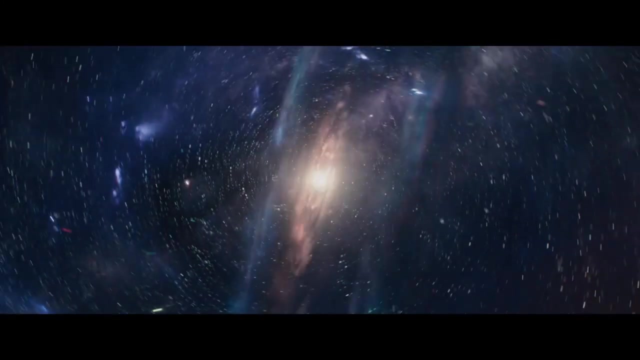 brain. our concept of time would cover just one cycle of the universe, with one big bang followed by another and another. This vision is both thrilling and humbling. There might be much more to space and time than we've thought and what we consider. everything might be just a small.